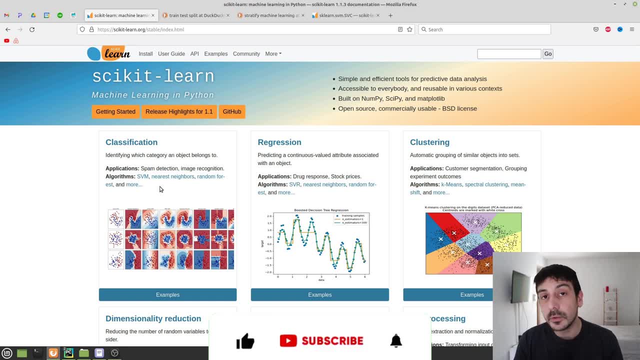 learning related problems, and if you want to work with computer vision or with machine learning, you will definitely need to be familiar with SeekItLearn. So this will be a very good example. this will be a very good opportunity in order to get more familiar with SeekItLearn. 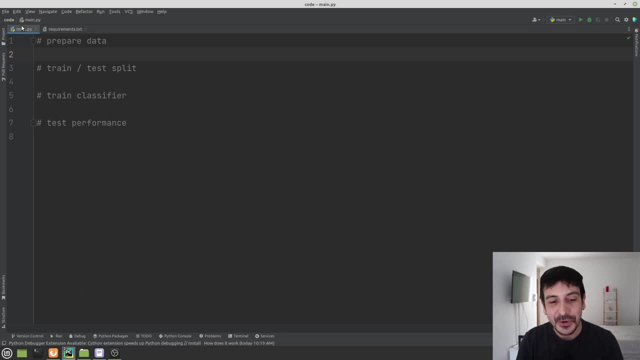 Now let's start with this project. Let's start with this tutorial, and the first step is preparing the data we are going to use in order to train this image classifier. And now let me show you the data we are going to use in today's tutorial. This is the data we are going to use. You can see. 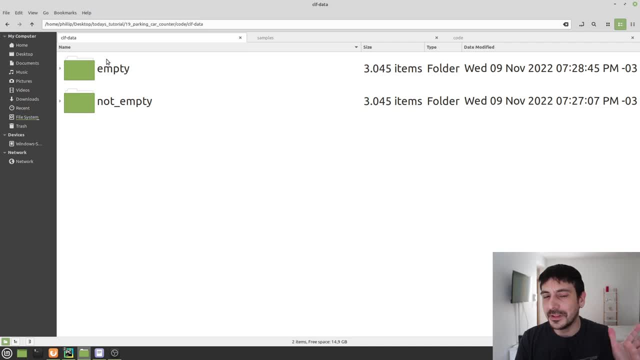 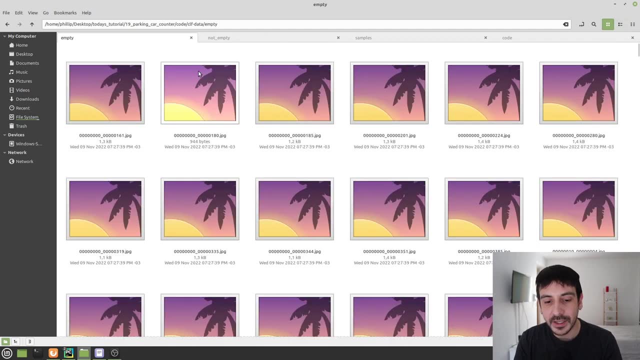 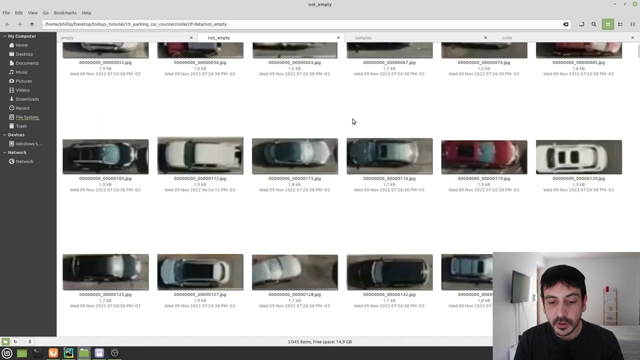 we have two different categories. The categories are empty or not empty. This sounds very strange, but let me show you exactly how these two categories look like, or how the data in each one of these categories look like, And you can see from the not empty category we have something that looks like this: So basically, we have cars. These are images. 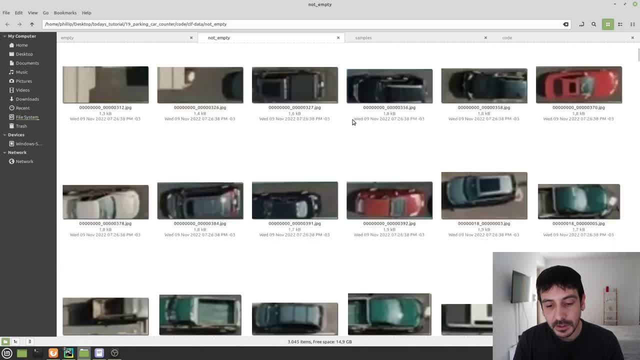 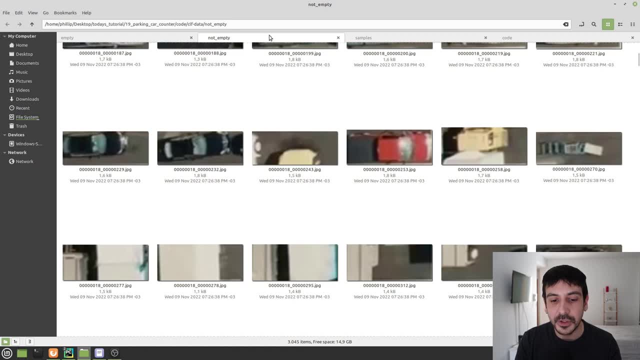 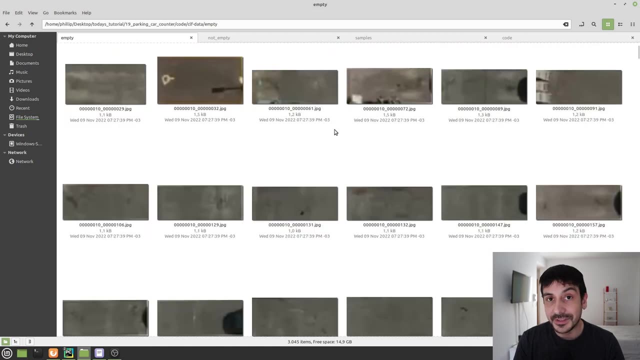 from cars and if I show you the, if I show you many, many different pictures, you can see that in all of them we can see pretty much the same situation. It's like a car. That's basically the not empty category. And then if I show you the empty category, this is pretty much an empty something. 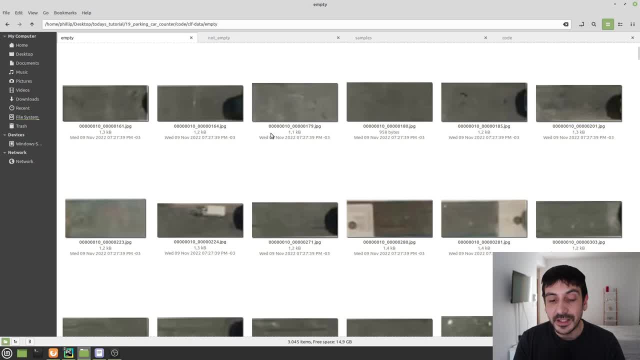 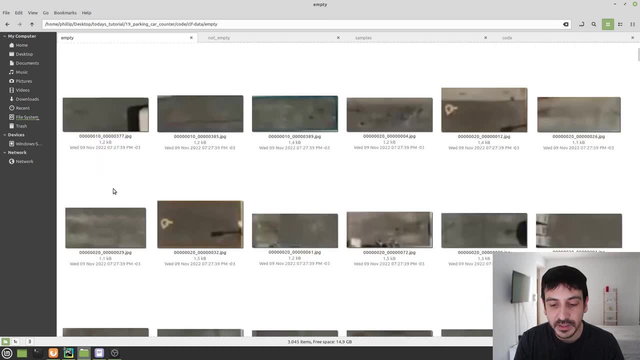 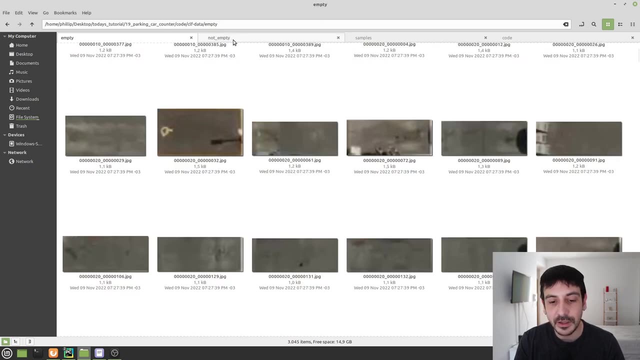 This is pretty much all images containing emptiness, Containing a completely empty. these are completely empty images. In some of them, they are very small objects, but you can see that all of the images are mostly empty, And these are how these two categories look like. This is how these two categories look like And this data comes from one of my previous. 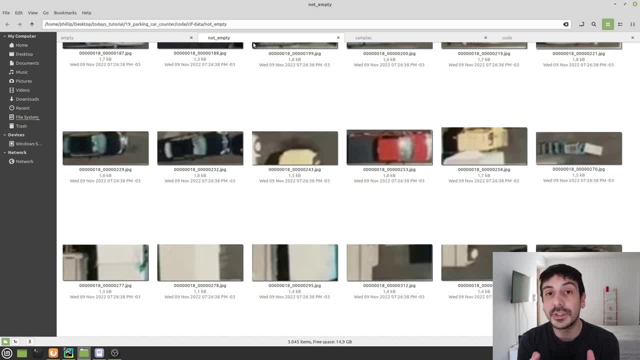 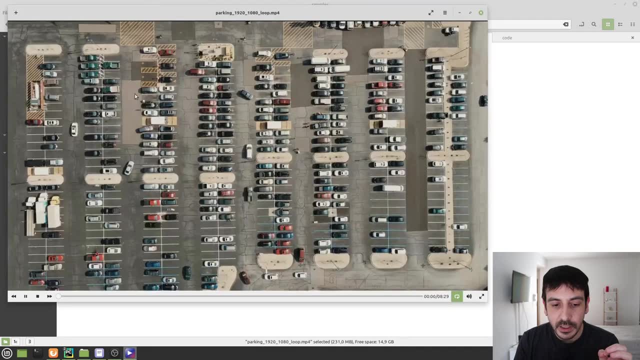 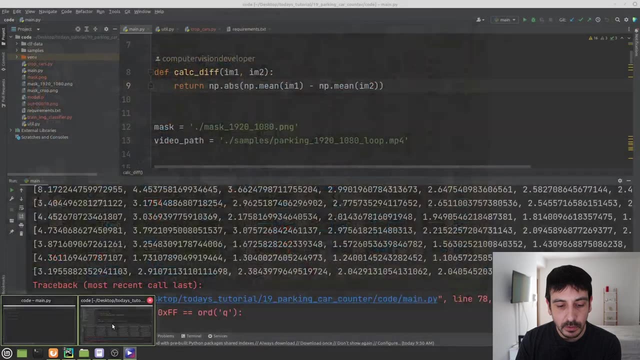 videos where I show you how to create a parking slot detector encounter using python and computer vision. In this other video, I show you how to take a video exactly like this from a video from a huge parking lot like this, and to make it look like this. Let me execute the code. 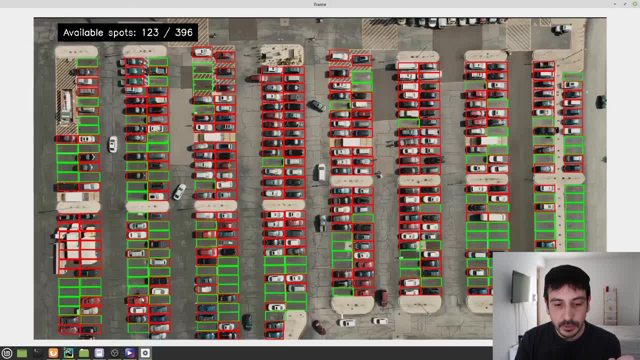 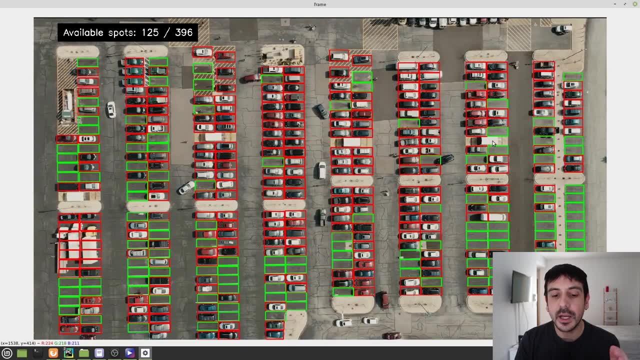 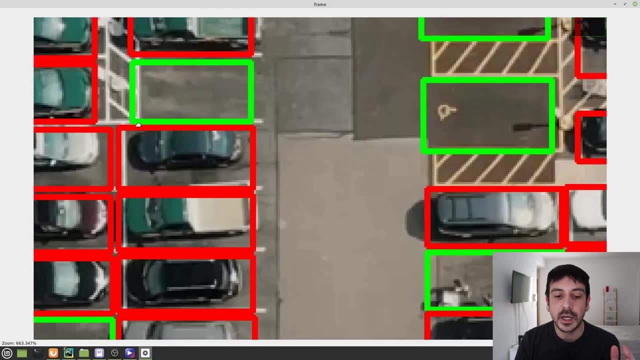 I show you how to build in this tutorial, and the idea was to go from here to here. The idea was to build something like this, where we detect absolutely all the parking slots and for each one of the parking slots, we classify if the parking slot is empty or not, and if it's empty, we plot it in green. 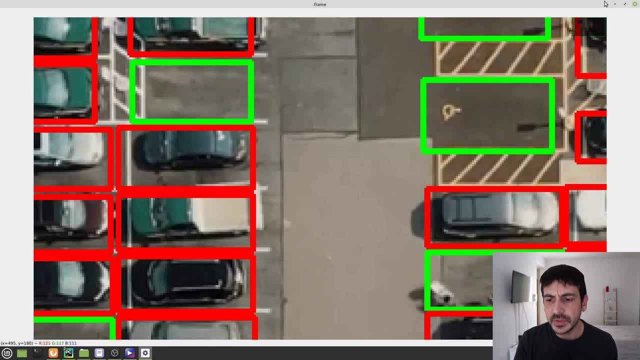 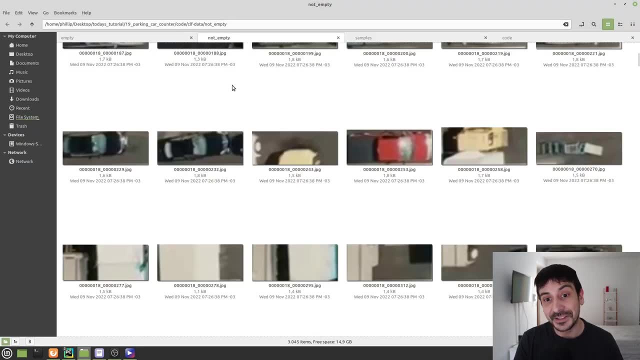 and if it's not empty, we plot it in red. So this is exactly where the data comes from, The data we are going to use in today's tutorial. You can see that for the not empty category, this is how the data looks like. These are images from parking slots containing cars and from the 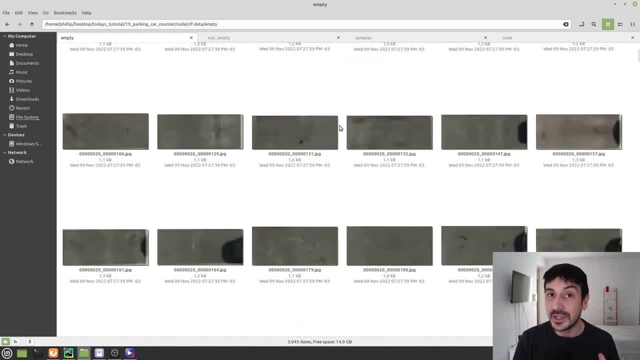 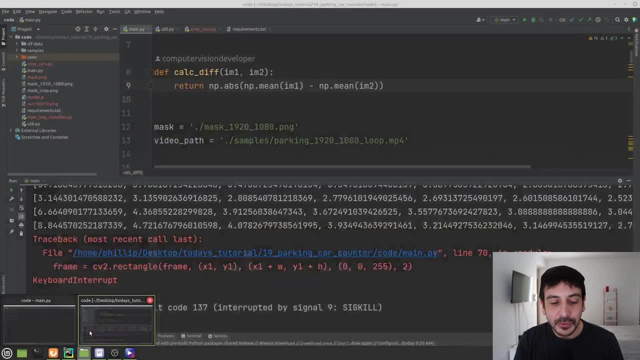 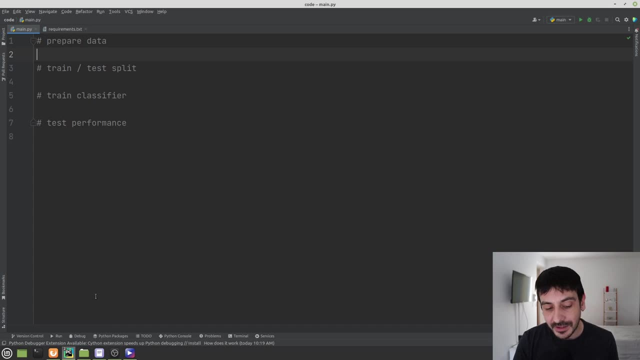 empty category. we have images from parking slots which are completely and absolutely empty. So this is the data we are going to use today and the image classifier I'm going to show you how to build in today's tutorial. it's a very robust classifier in situations like this. in situations 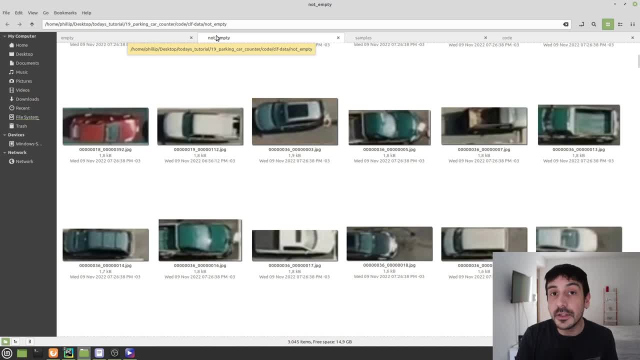 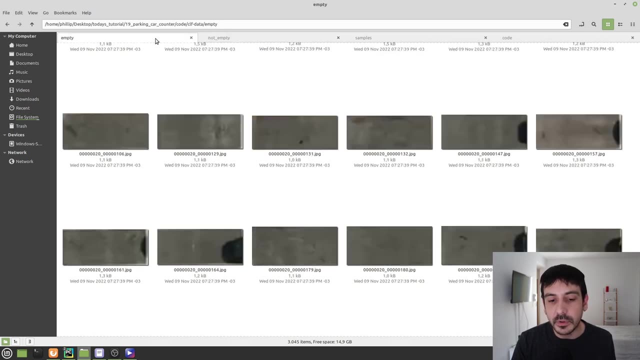 where the data we have in situations, where the classification we want to make on our data, it's very easy, it's very simple. right where the different categories we want to tell apart, the different categories we want to classify, they are visually super, super, super distinct. they are super different. right, in this case, we have images from cars and 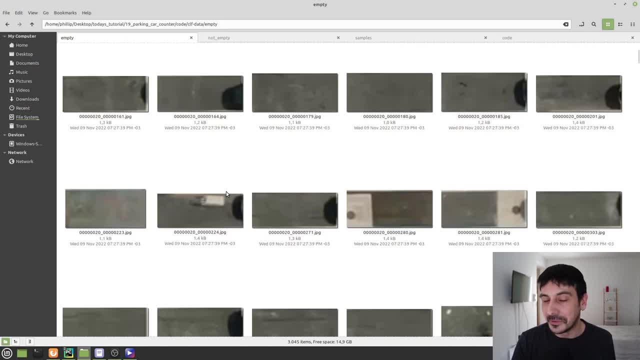 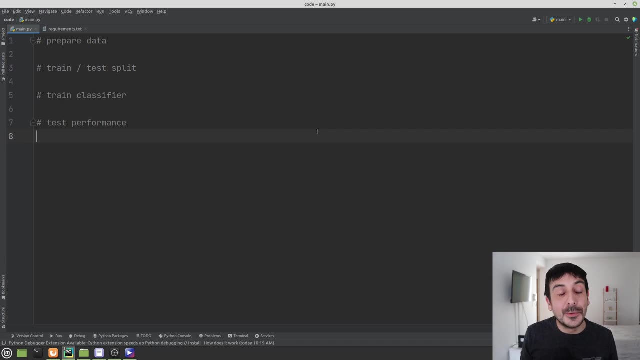 in the solar category, we have absolutely empty images, right? the image classifier i'm going to show you today. it's very robust and it works super, super well in situations like this, and the reason i'm saying this is because this may not be a state of the art image classifier if you look for papers. 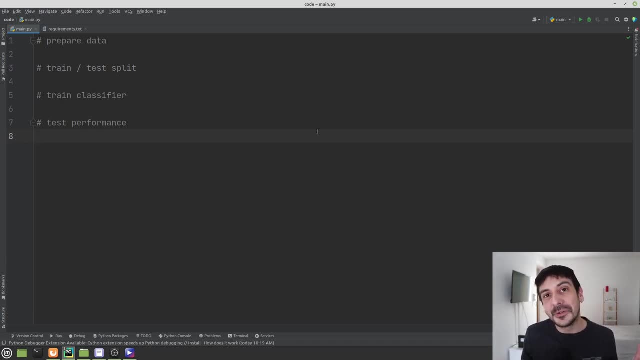 or if you look for the most recent techniques, obviously you are not going to find the classifier we're going to make today. we're going to build today and it's big and it's definitely not the most robust classifier in in in the machine learning industry. but if you want to solve, 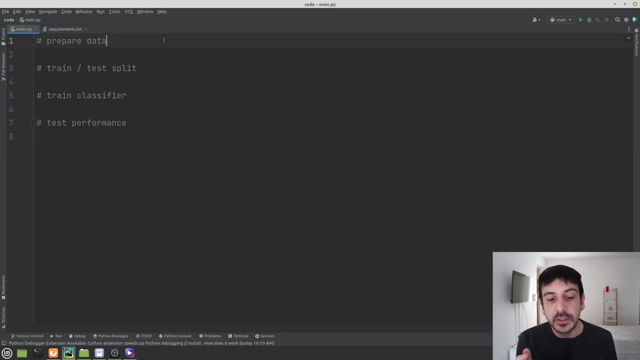 like a very, very simple problem like the one we are going to solve today. this image classifier will be more than enough, and i'm going to show you exactly what's the performance we achieve with this classifier, but that's later on in this tutorial. now let's get started. i already 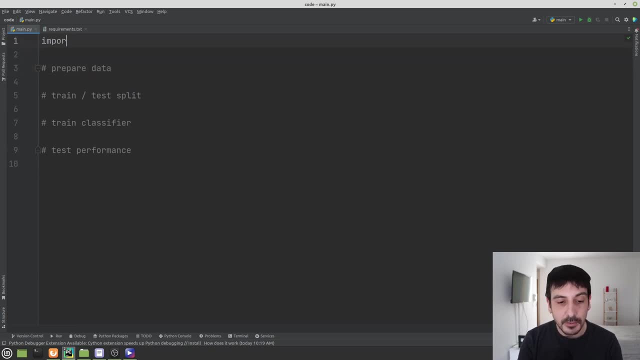 show you the data we are going to use. and the first thing i'm going to do is to import os, which is a library which we definitely need in order to work with data and to read data and to load data from our computer. so i'm going to define a directory which is input directory and in this 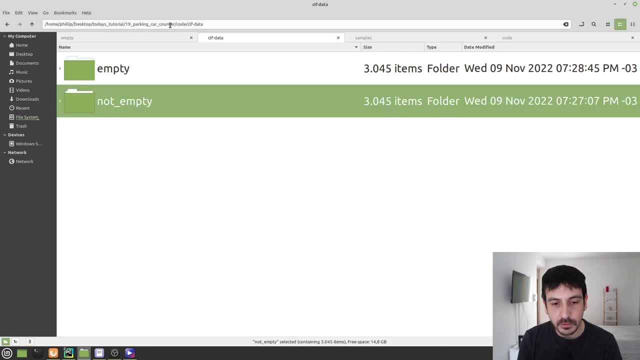 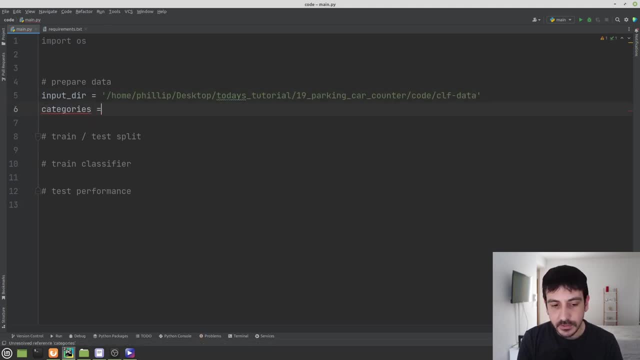 case, i'm just going to hard code where the input directory is located, which is here. this will be something like this: and then i'm going to define our categories, and i'm also going to hard code. it says something like this: or categories are empty and not empty. okay, and then the only thing i'm 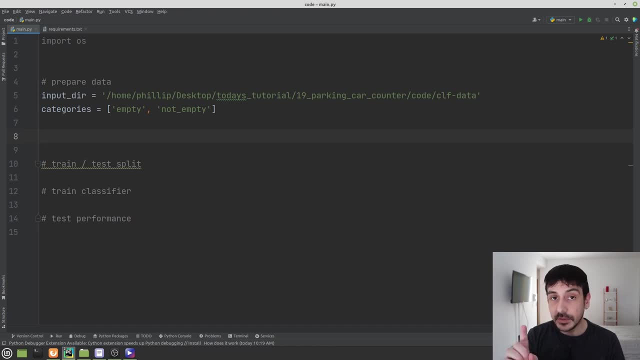 going to do is to define two lists, which are the list, which are going to contain our data. one of them will be data and then the other one will be labels, and i'm going to show you exactly how we are going to use these two objects later on this tutorial. and now what we're going to. 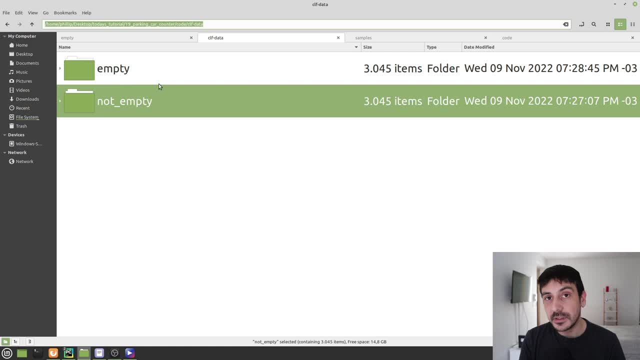 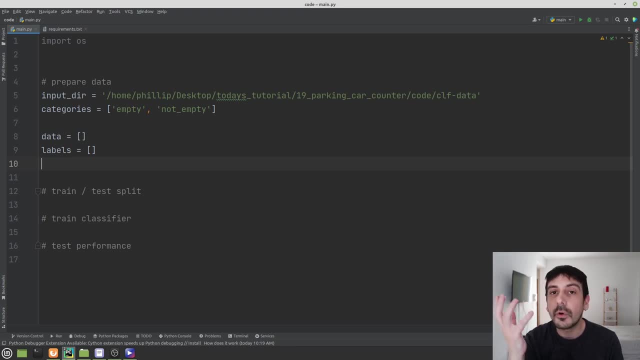 do is to iterate in absolutely all the images in this classifier and then we're going to add two directories and we are going to load these images, we are going to read these images and we are going to format these images, this data, in a way that fits well the classifier we're going to 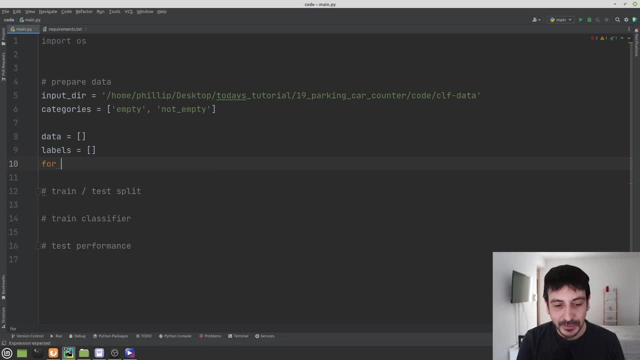 use later today. so let's start with it. i'm going to say something like for category in categories and then for file in something like os list, dir, input, dir, and then i'm going to define the image path like os path, join, and then input directory and category and sorry, this will be. 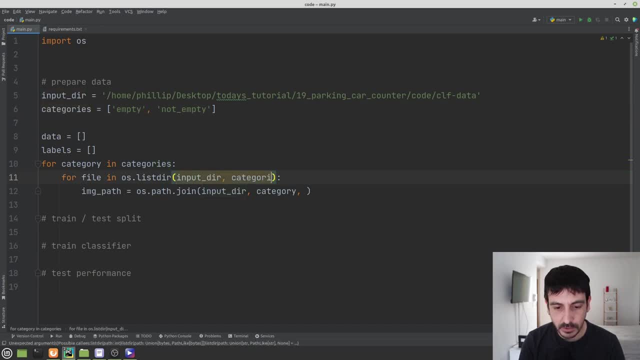 os, dot, pad dot. join input, dir and category. okay, because we are working in absolutely all the files for each one of our categories, right, something like this: okay, image path, join input, dir, category and then file, and then we have defined exactly what's the location of our images. 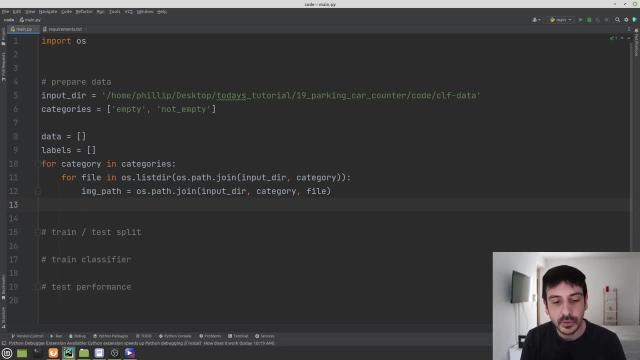 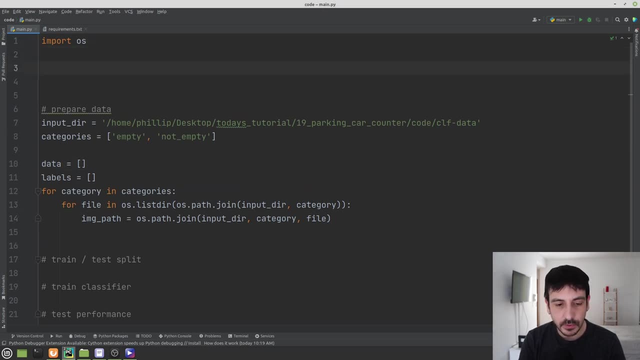 now the only thing we need to do is to read our images and to save our images into this list. so, in order to read our images, i am going to import from skimageio, import in, read in this channel in all the videos i have made so far. 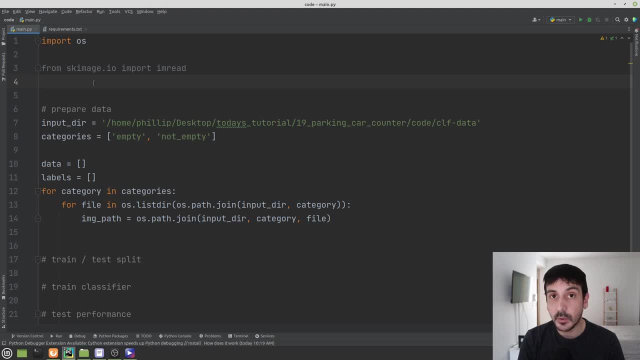 we usually used opencv as an image processing library and obviously opencv- it's by far the most popular and the most comprehensive of all image processing libraries- is the one i use the most in my projects. but there are also other libraries which are more convenient in different 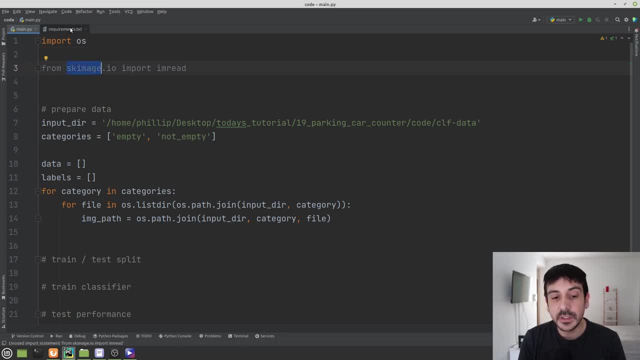 situations and, for example, in this case, we are going to use ckit image. we're going to use this image processing library in order to read the images from our disk, from our computer. so i'm going to call in read from image path and this will be image. okay. 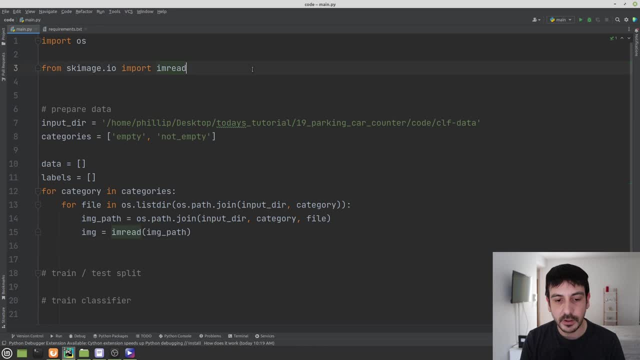 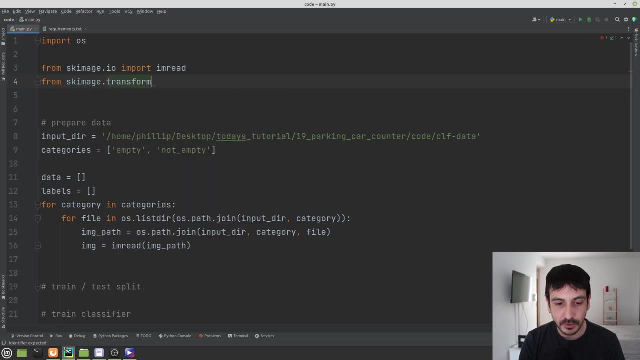 and now i'm going to resize this image and for that i am going to import another function from cgd image which is called from cgd image: dot transform, import, resize. so i'm going to call resize, i need to input my image and i need to input the new size. 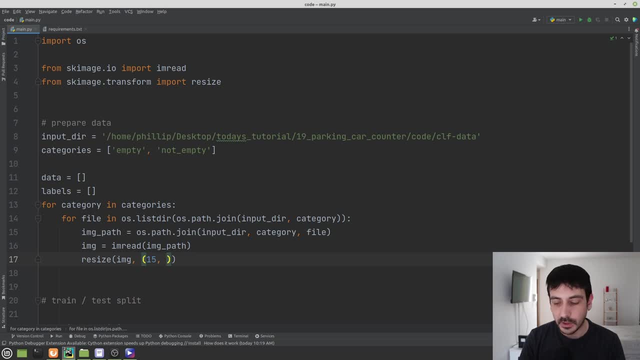 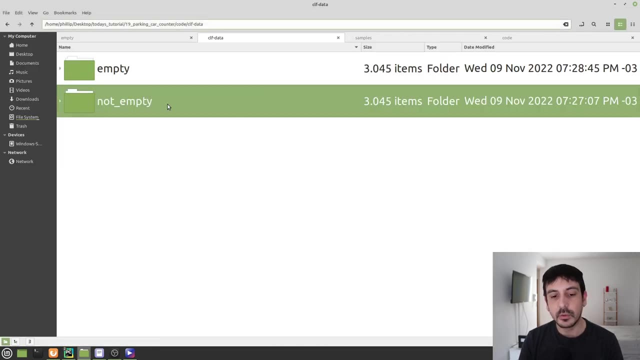 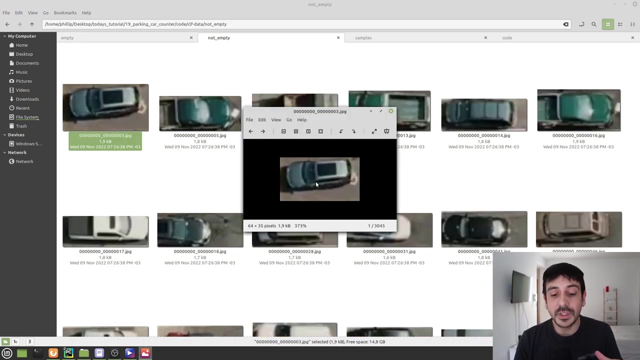 which the the new size. i'm going to resize all my images too, which is 15 times 15, and this will be my image. so i'm walking through absolutely all the images in these two directories. i'm taking these images, i'm reading these images from my computer and i'm resizing these images from this size. 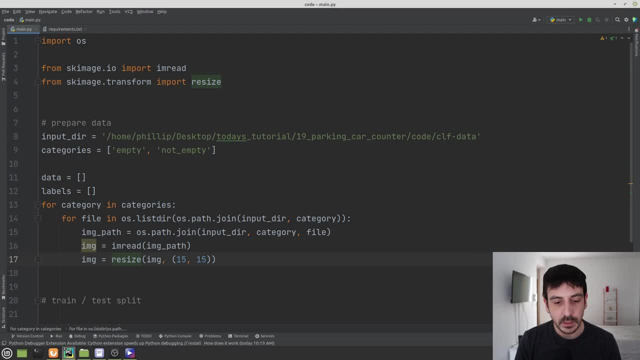 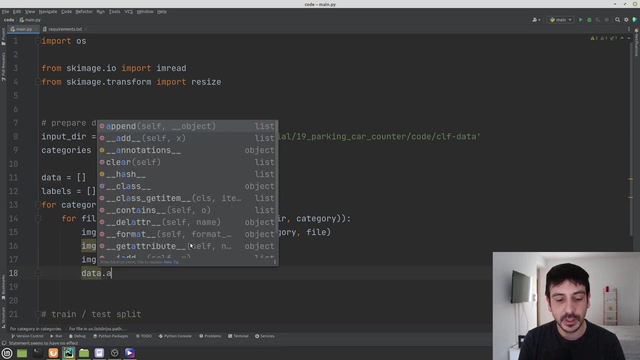 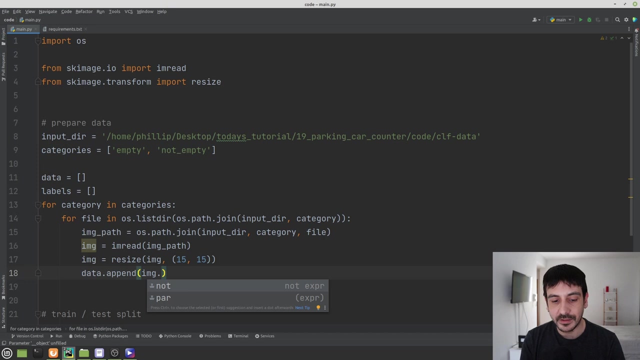 to 15 times 15.. okay, now let's continue. i have resized all of our images and what i need to do now is to append this data into the lever, into the list i have created in order to contain all my data. so data dot append and we're not going to append the image like the, the, the image we have read and 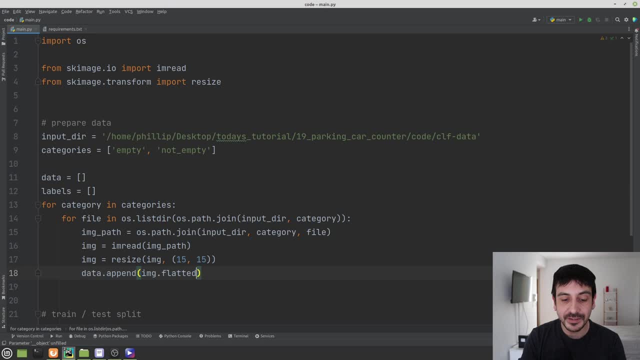 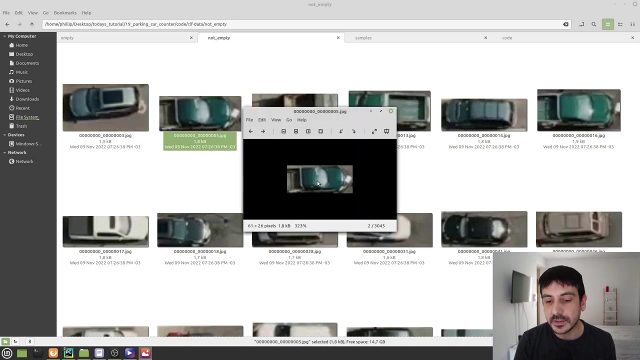 we have resized, but we are going to append the flooded image. we are going to take our image and we are going to make it into an array, right, because currently our image is something like a, like a matrix, right, it's something like, uh, like, a matrix of size, for example, in this case, 61 times 26. 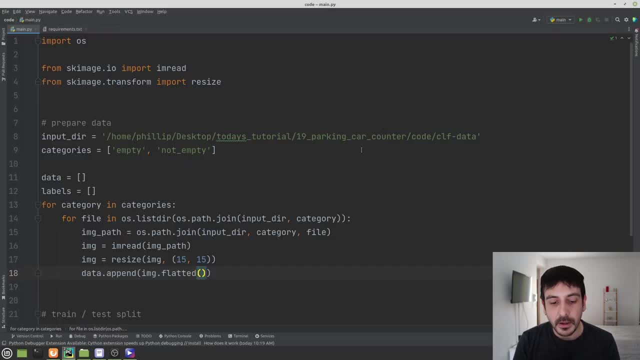 and three channels. bg, it's bgr. we have recited this image. now it's 15 times 15 and three channels. now we want to take all of that information and we want to make it into only one very, very long array. right, we want to make it unidimensional. so that's why we are calling flutter. 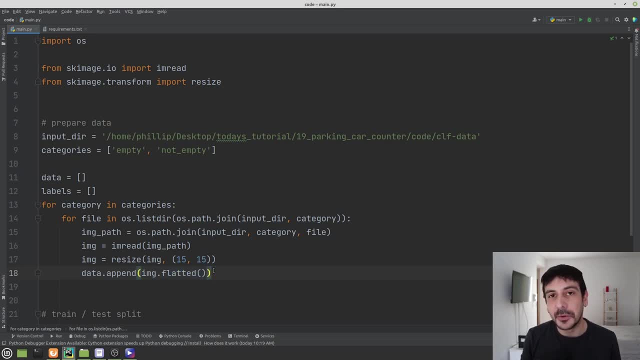 and the reason we are doing this is because that's what we need to do in order to use the image classifier we're going to use today. when we are working with machine learning, you will notice different classifiers and different models and different libraries and different, so on different everything, require different uh formats or require we format the. 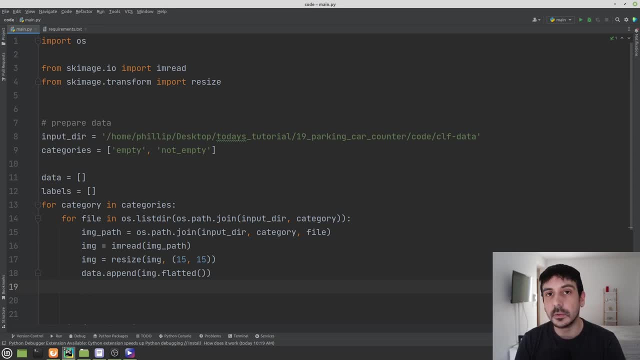 data differently in order to be fed into the machine learning model, into the classifier or into the, whatever we are using, and in this particular case, we need to flood the data. we need to make the data into an array before we input this data into our classifier. so that's all for the data, and we also need to append the category for this data, the label. 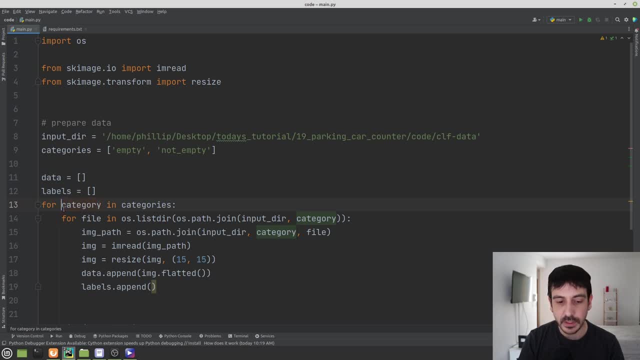 and in order to that, i'm going to walk through the categories slightly in a slightly different way. i'm going to call this category index- category in enumerate categories, and now i will append category index to these. labels are right to this label list and that's pretty much. 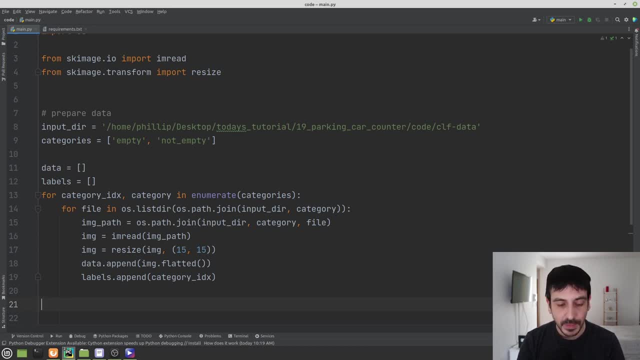 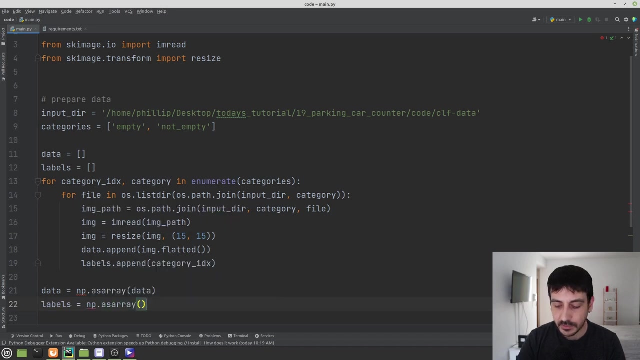 what we need to do. the only thing i'm going to do next is to uh, cast each one of these lists into a numpy array, so i'm going to say as a right, and then date okay. and i'm going to do the same with labels mp as a right, labels. i know what you're thinking. hey, felipe, it is not going to work. 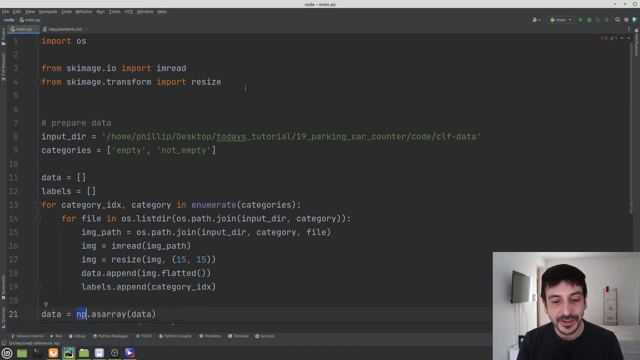 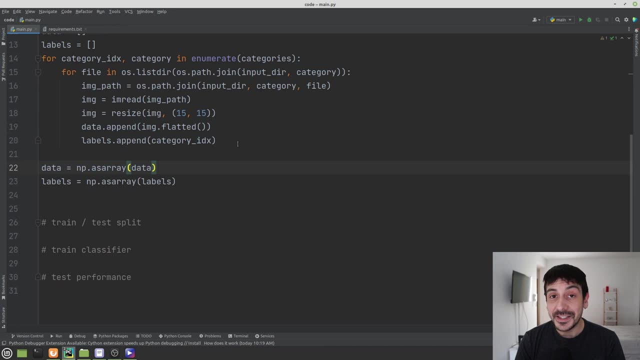 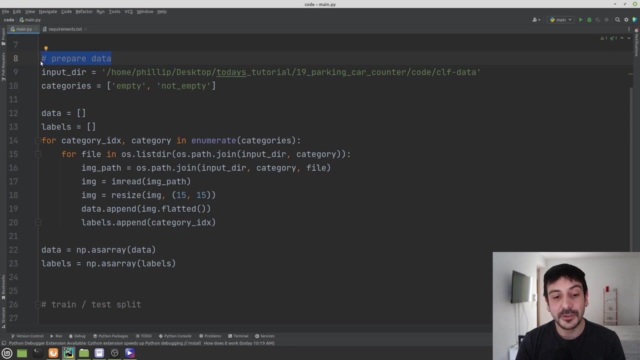 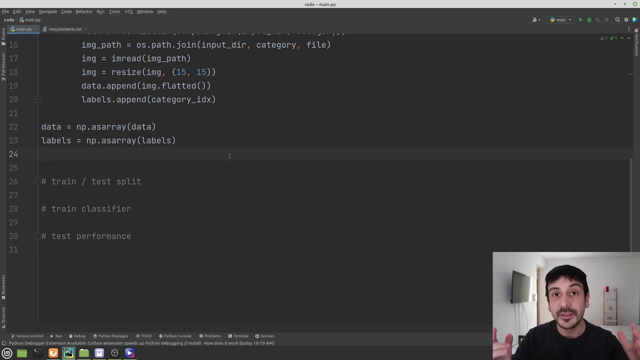 because you have not imported numpy, and you are completely right. so i am going to import numpy now. import numpy as np. okay, so that is it. that's all we need to do in order to load our data and in order to prepare our data to be fed into the classifier or in order to move to the next step. that is it. we have completed the. 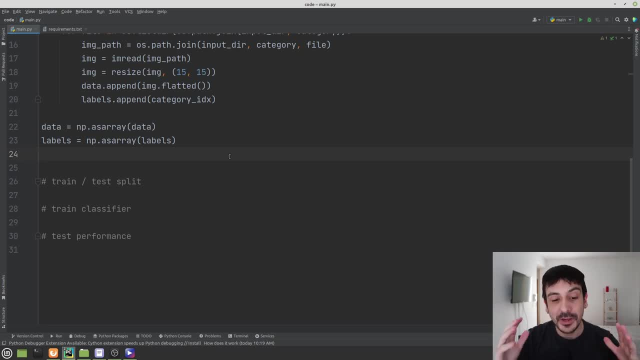 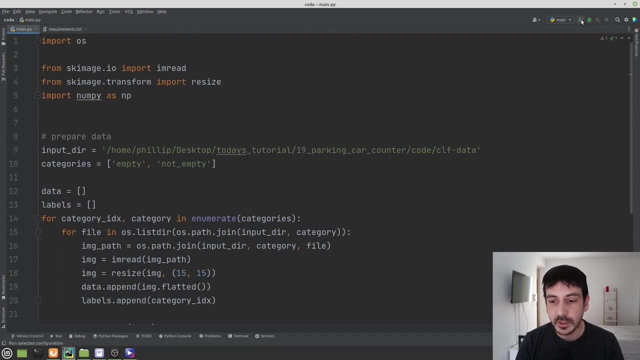 first step in our process. so congratulations. we are one step closer to reach our goal of training or image classifier. now, in order to make sure everything works properly and we don't have any error, i'm going to execute the code as the image classifier. i'm going to execute the code as the. 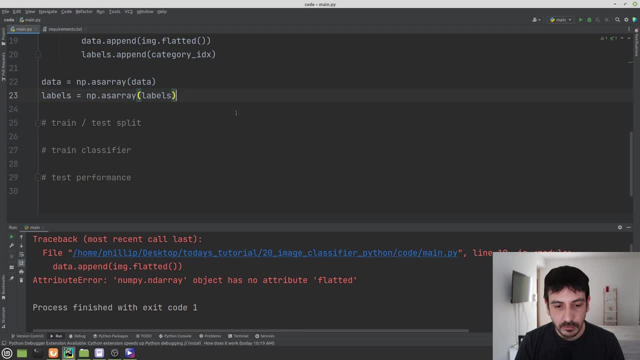 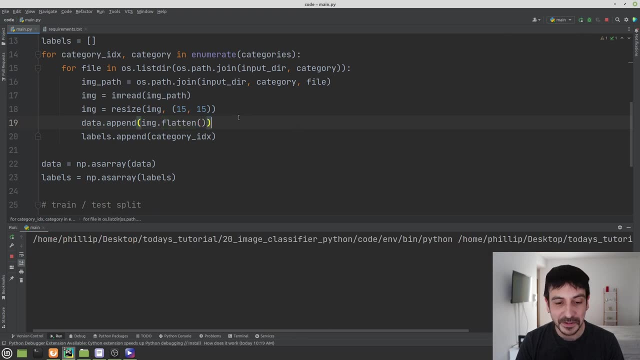 image classifier. i'm going to execute the code as the image classifier. i'm going to execute the code as it is now, and numpy has no flutter. maybe it's flatten. i think it's flat and maybe i made a mistake, so let's see what happens now. 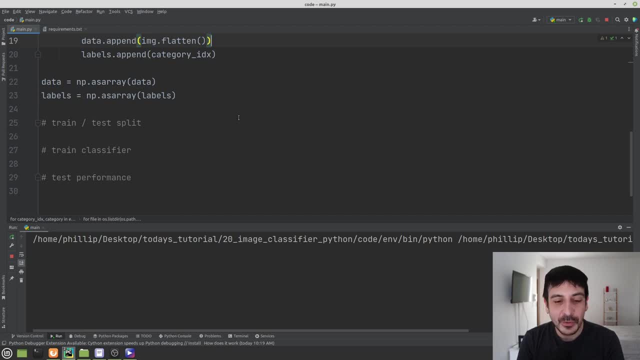 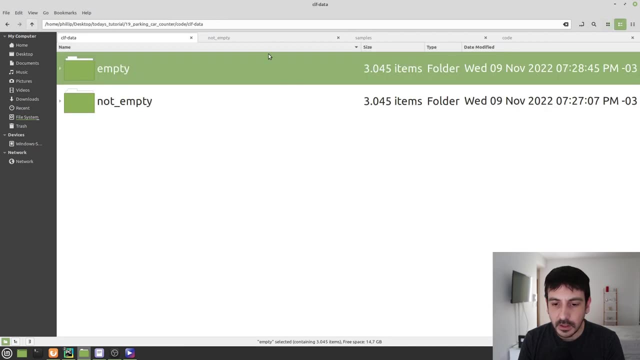 it seems we don't have any error. so, yeah, i made a mistake. now we have to wait a few minutes because, remember, we are walking through absolutely all the images in these two directories and we have, among the two directories, we have 6090 images. so this is going to take some time, but yeah. 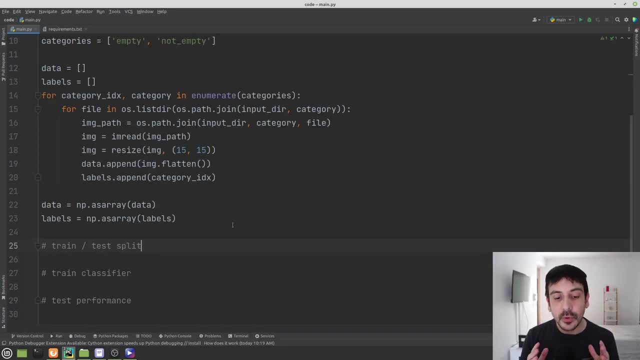 it's going to take some time, but yeah, and now it's time to move to the next step, where we are going to split our data into two different sets. we are going to create a training set and we are also going to create a test set. the training set is the one we are going to use in order to train our image classifier. 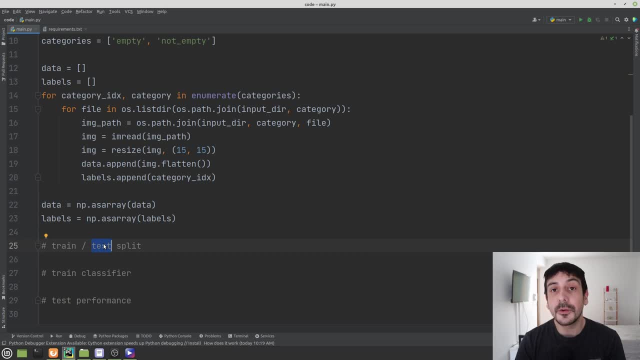 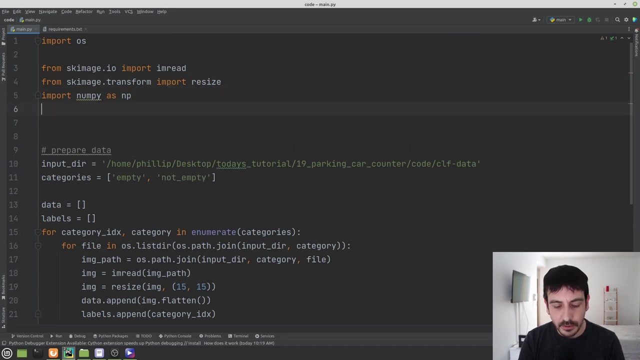 and then the test set is the one we are going to use to test the performance of the classifier we are going to train. so we definitely need to split all of our data into these two sets and this is the function we are going to use. we need to import another function from cgit: learn. 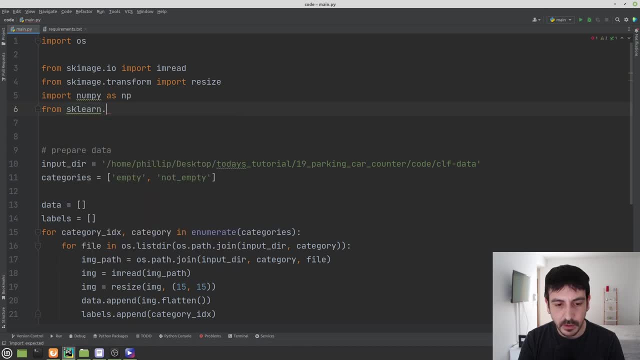 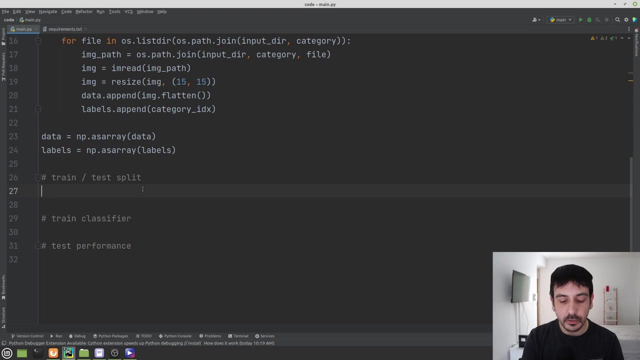 and this function will be something like from cgit learn dot model selection, if i'm not mistaken, import train test split. yeah, so this is how i'm going. we are going to use this function. i'm just going to write some things and then i'm going to explain it, so this will be something like x train. 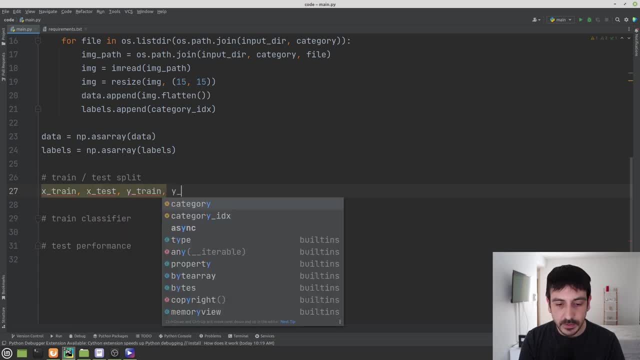 x test, train y test, this calling or data x and y. it's a very popular convention in machine learning, so we are going to do it too, and this will be our train test split function, and we need to input data labels, and then there will be other parameters as test size. i'm going to set this in. 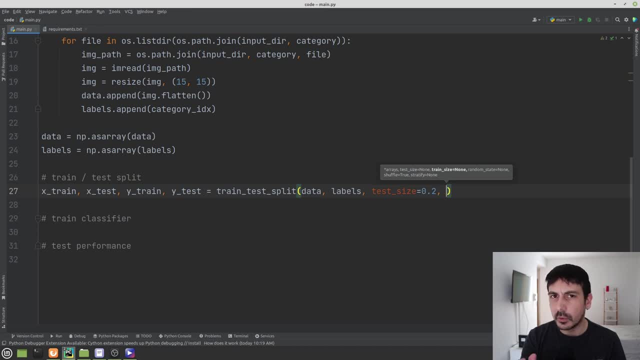 20 in 0.2. don't worry, i'm going to explain exactly why i'm setting all these parameters, you know in a couple of minutes. then another parameter is stratify. this will be according to labels, and then shuffle. i'm going to call shuffle here and this will be true. okay, so i have called train test. 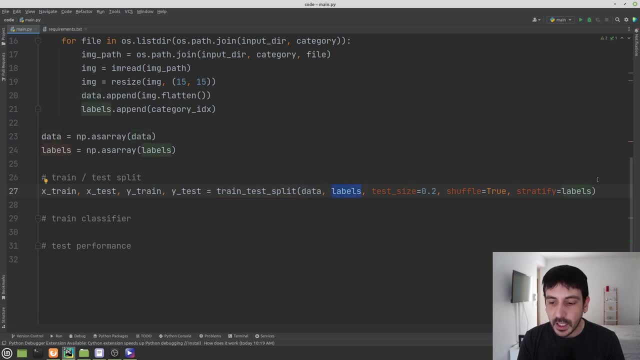 split. i have input or data and or labels, and then i have specified a few parameters in order to show you exactly what these parameters mean. uh, i'm going to start with test size. i told you we were going to set the data into two different sets: the training sets. the train set and the test set. now, 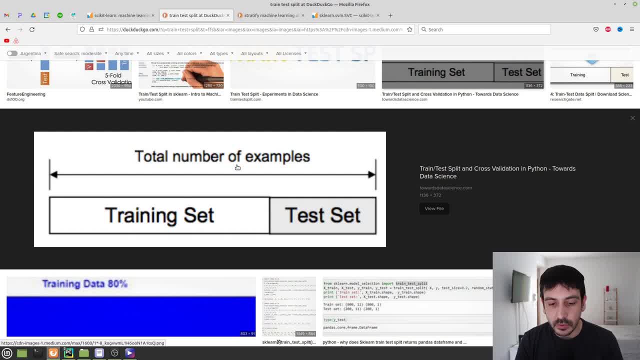 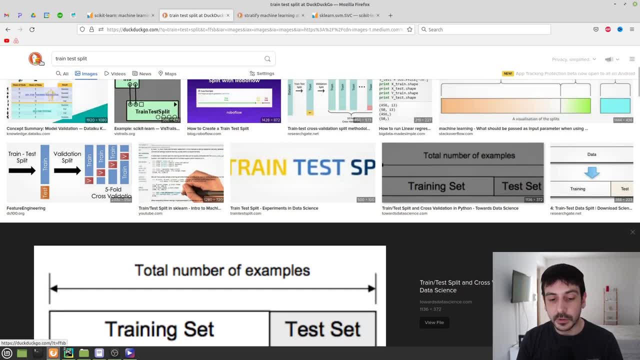 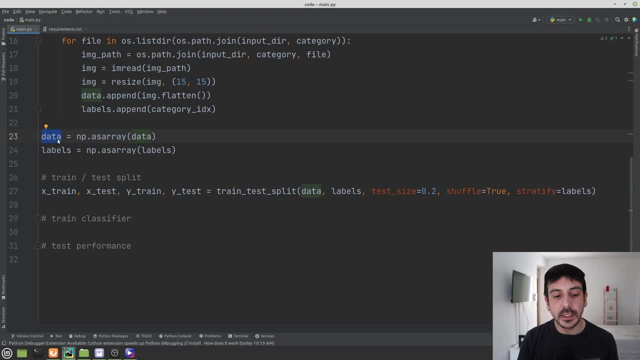 let me show you an image to show you more um what, what this means, to show you exactly how this looks like. so this is an image i found online, this is an image i found on google, or actually on docgov, and basically you can see that we have an array which is called data, which contains all of our 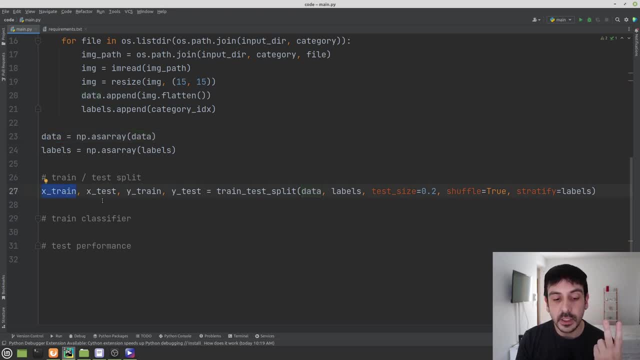 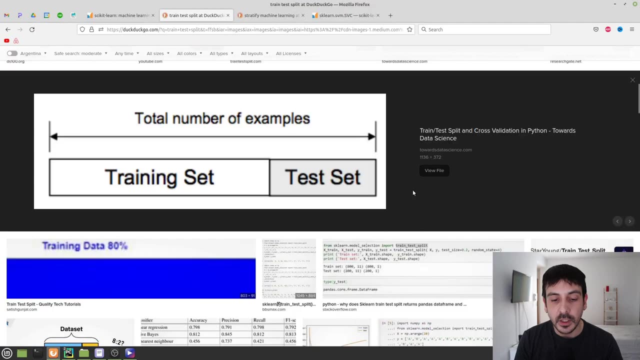 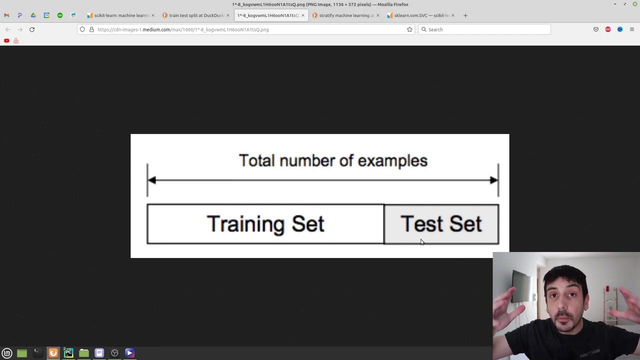 data and we are creating two different arrays from it. we are creating x- train and x- test, and we are specifying this size, this split size, which is 0.2. so what we are doing is creating two different sets, which are training set and test set, from the total amount of our samples, from. 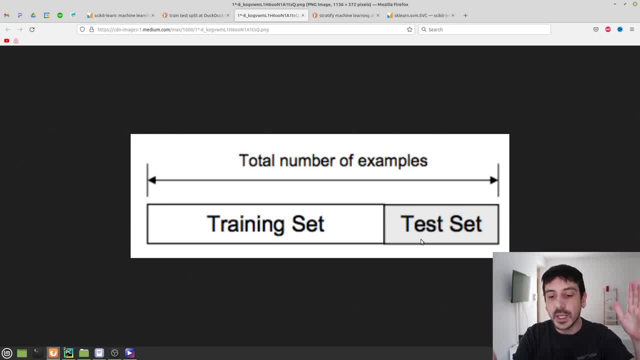 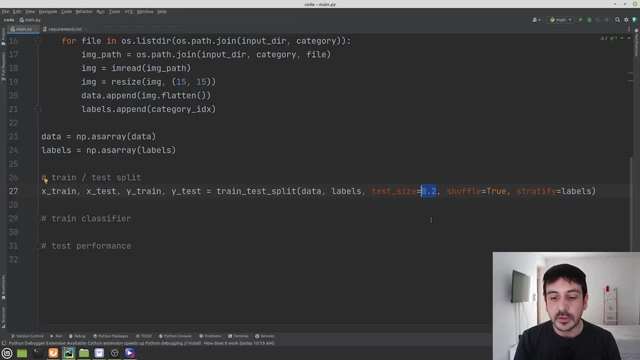 all of our data. we are splitting all of our data into two different sets and the way we decide what's the size of the test set is by specifying this parameter. so currently we are telling train test split to make this split in a way that 20 percent of followers of all of our samples are in the test. 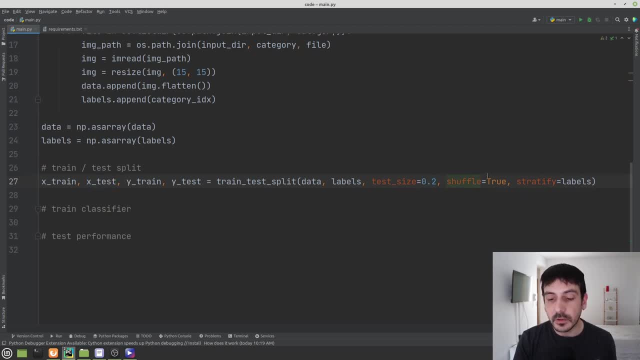 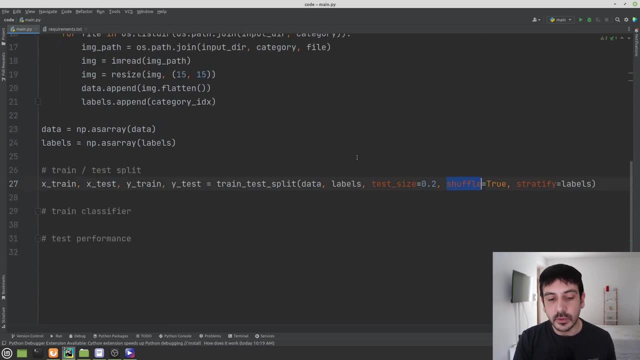 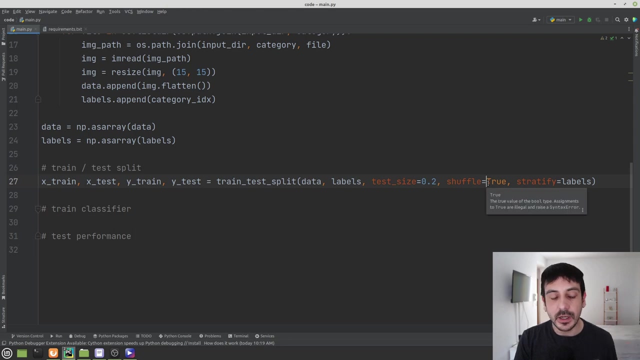 set right now. moving to the next argument: shuffle equal. true, this is something that we always want to do when we are creating data, when we are preparing data in order to be fed into a machine learning classifier. we definitely want to shuffle this data first, so we can avoid absolutely every. 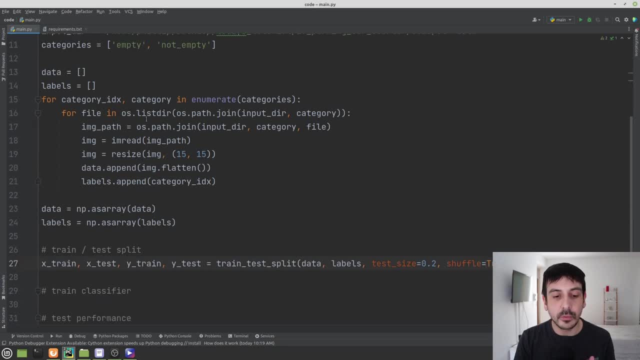 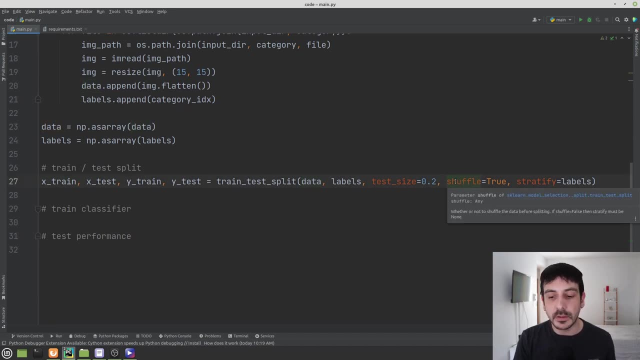 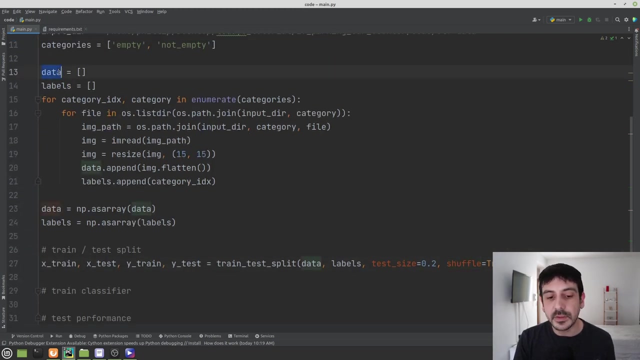 bias we had when we were reading the data, when we were creating the this data arise. we definitely want to shuffle the data first. this is a very good practice. sometimes there are some biases which we are not aware of. sometimes the way we are reading the data or the way we are creating these arise we we are making some mistakes or we are. 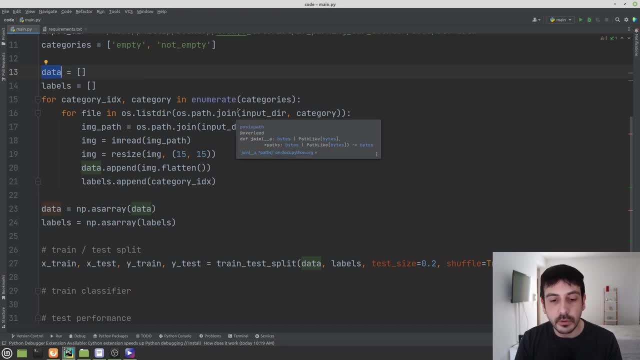 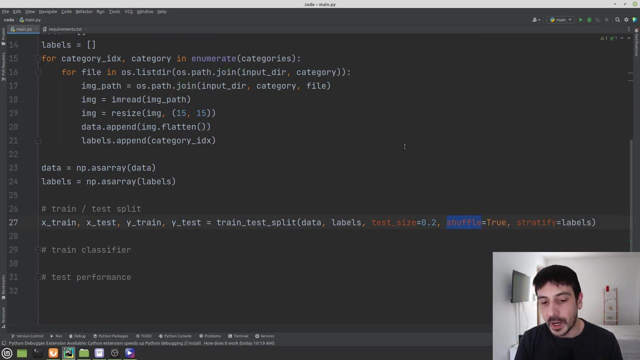 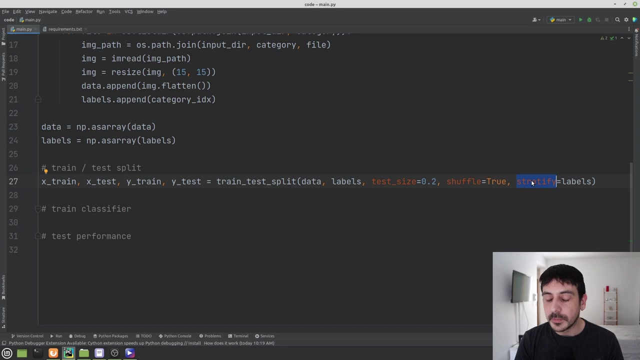 i don't know the way this working is done. maybe it's a alphabetical order or maybe it's whatever. we always want to shuffle the data first. that's a very good practice to avoid any type of bias when we were reading the data and creating these arise. then stratify equals labels. i will say it's always a. 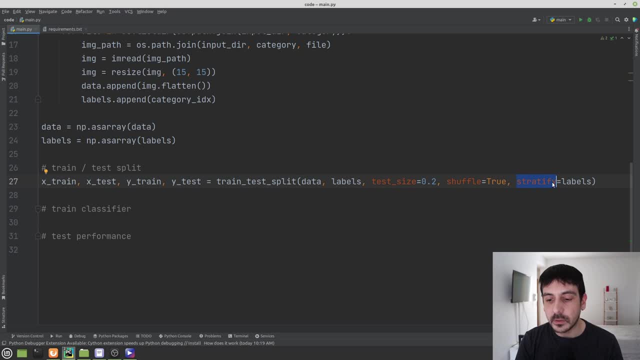 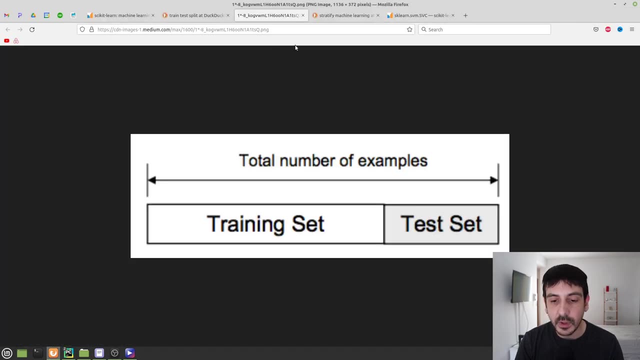 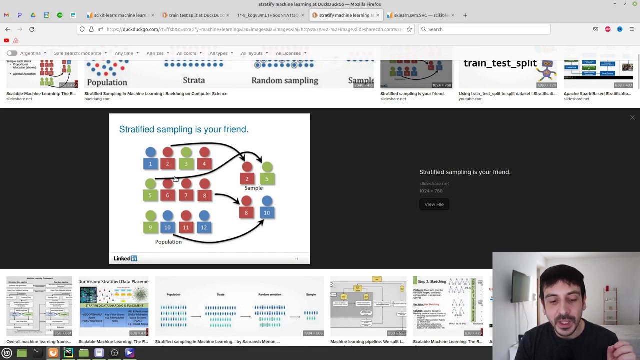 good practice when we are splitting our data into two different sets. to define exactly how we are stratifying this uh split, and in order to show you exactly what stratify means, i'm going to show you this picture, which i also found online on duckduckgo, and basically you can see that we have a data set. 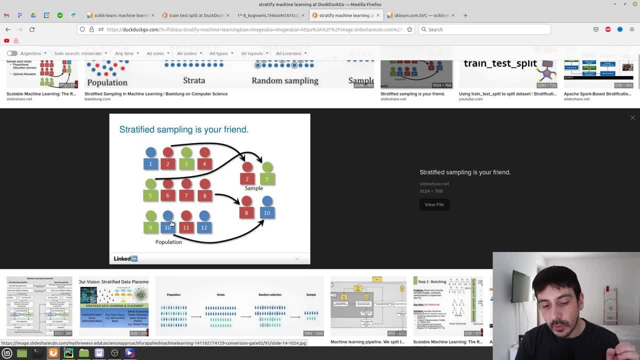 people and you can see three of these people are blue, three of these people are green and then six of these people are red and in this example we are taking a sample of four elements of four people, and the way this sampling is done is by stratifying by the different labels. so if you look at the 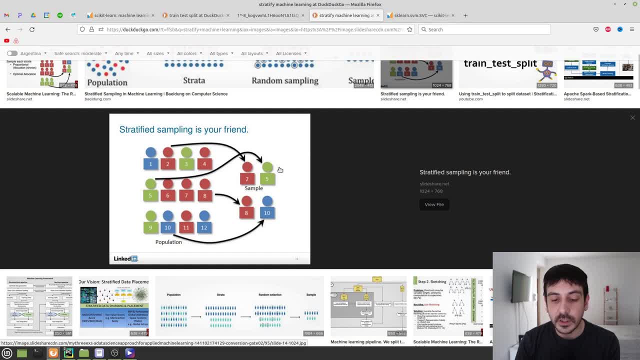 sample. you can see that two of these samples are red, one of the samples is green and the other one is blue, so we are keeping the same proportion of the different labels in our original data set. that's exactly what we are doing when we are stratifying according to the labels. it's like a 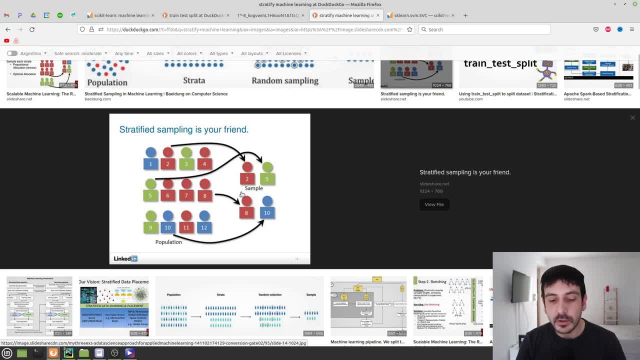 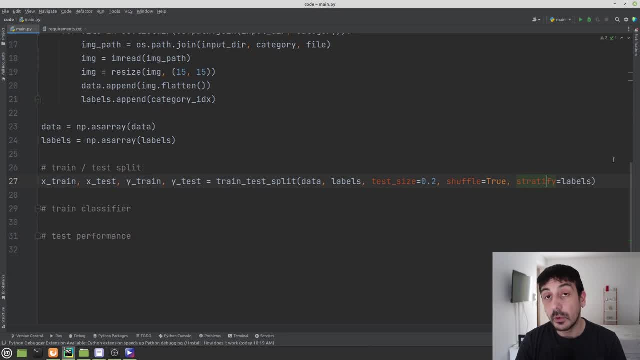 way to make sure that the all the different labels are going to be in exactly the same proportion as in the original data set, so it's definitely a good practice. this is something we always want to do. now let's continue, and you can see that we have completed the second step in our process. 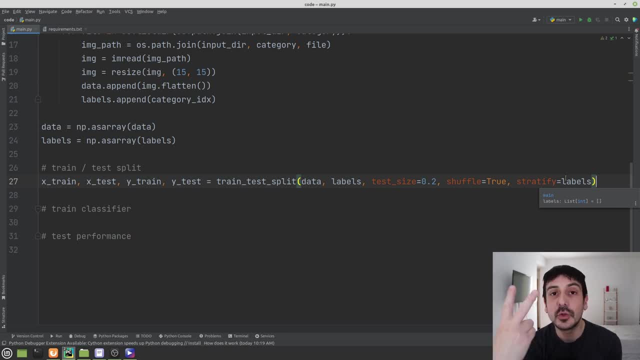 we are one step closer. we have only two steps left, two steps to go. we are one step closer of training or image classifier, and that's going to be all for splitting our data into a training set and a test set. now it's time to train or image classifier. now it's time to do like the, the actual training. 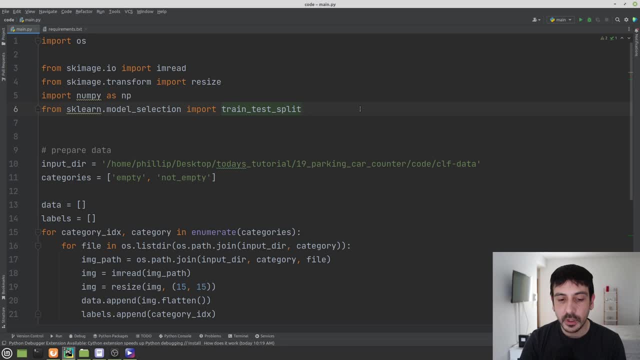 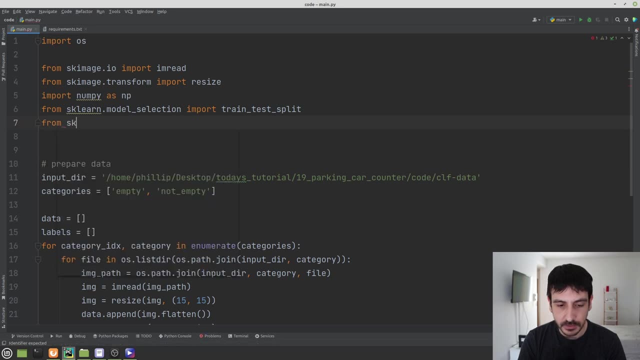 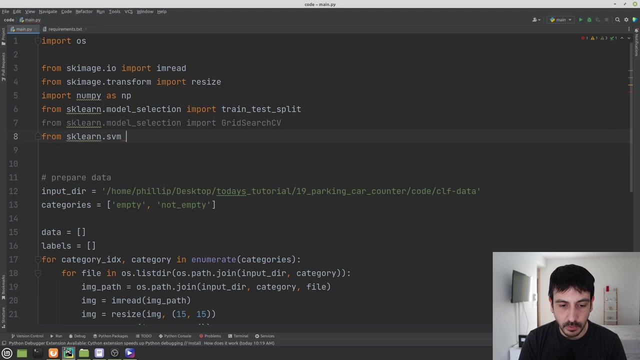 and this is how we are going to do it. i'm going to import another function which is called, if i remember correctly, from ski learn- i think it's small selection as well- import, uh, grid search, cb, and then from a skilearn that svm imports svc. okay, so 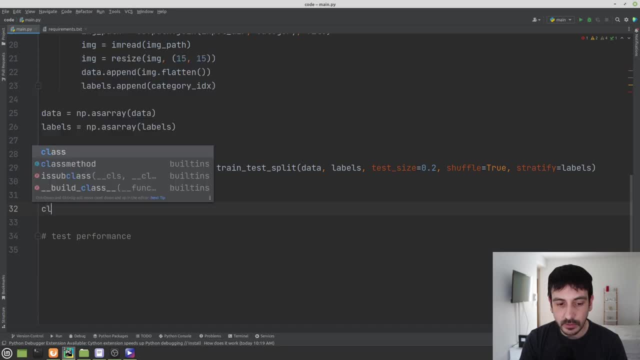 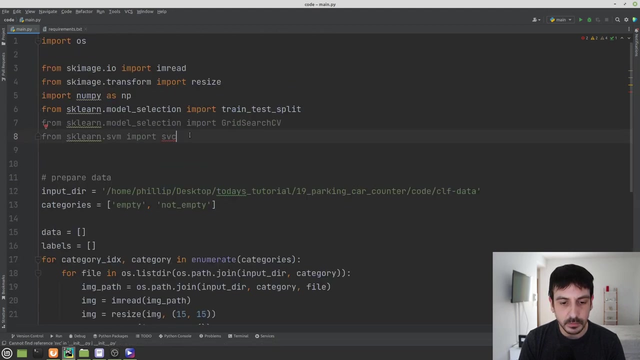 the first thing i'm going to do is to define a, an object which is called classifier, and this will be something like this: this is the classifier we are going to use. uh, it's svc. uh, let's see if it's okay. is killer svm sport? i think it's okay for. 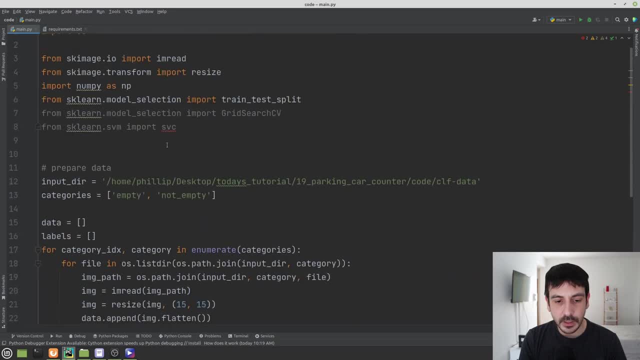 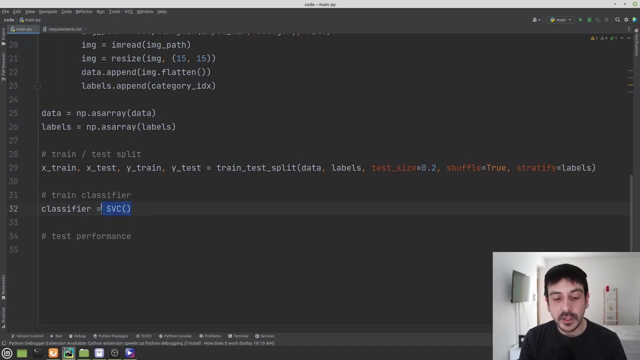 some reason it doesn't really found it. now i see what's the error: svc should be in capital letters and now everything should be okay, okay. so what i'm doing here is creating a new instance of this object and i'm calling this object classifier, and this is the classifier we are going to use. 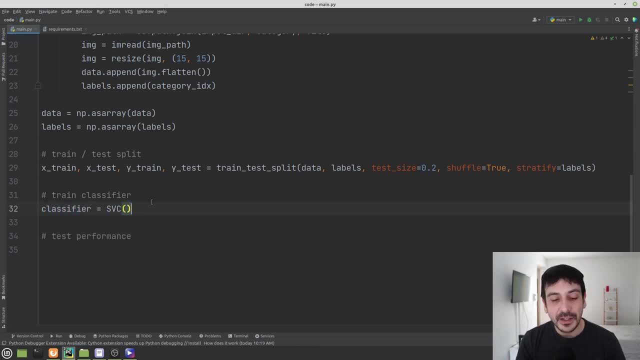 in order to train our image classifier. so what i'm going to do next is to define another object, which is parameters, and this will be something like this. i'm just going to write it and i'm going to explain it in a couple of minutes. i'm going to define something like a list of only one element. 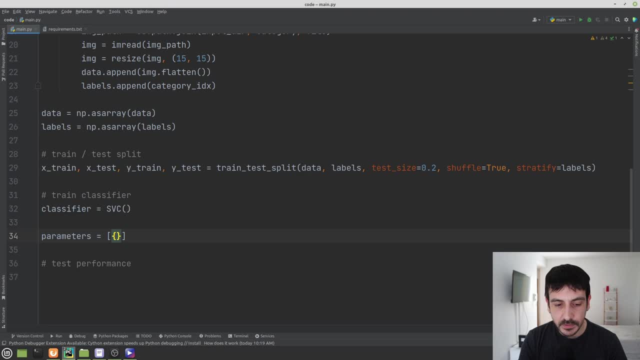 which is going to be a dictionary with two keys. one of these keys will be gamma, and then the other key will be c, and that's pretty much all, and then i'm going to define a list for each one of these items, and for gamma it will be something. 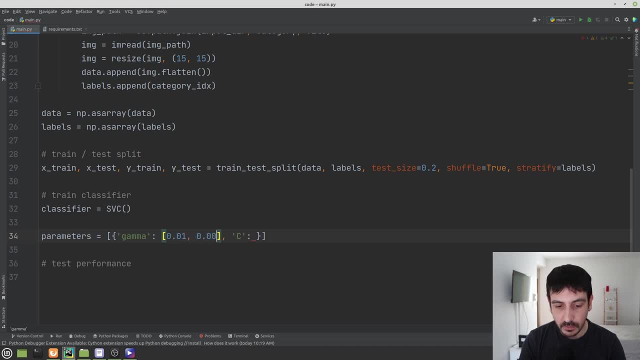 like 0.01, 0.001 and 0.0001, okay. and for c, i'm going to do something like 110, 100 and 1000, okay. and then i it's when i'm going to call grid search, i'm going to find a new object which is called. 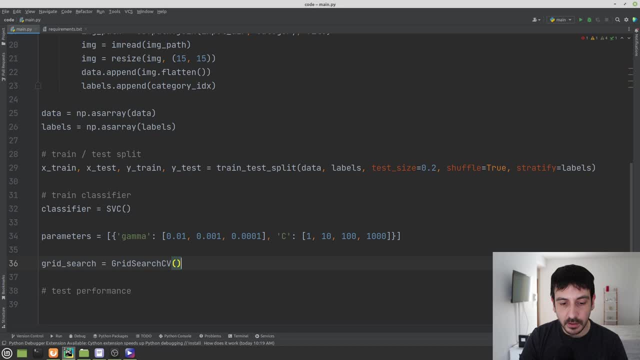 and this will be research cv, and i'm going to input my these two objects. i just created the classifier and the parameters, okay, and now let me show you exactly what i'm doing. i'm creating a new instance of svc and i'm calling this instance classifier. and this is the classifier we are. 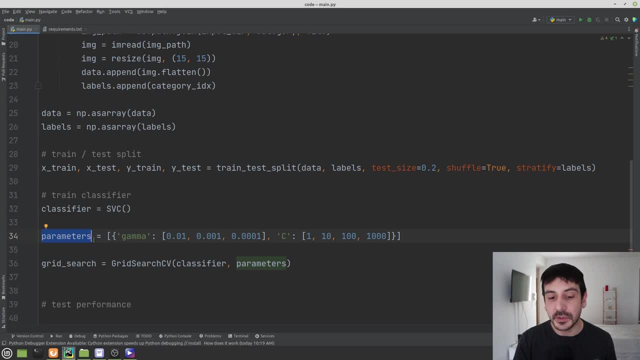 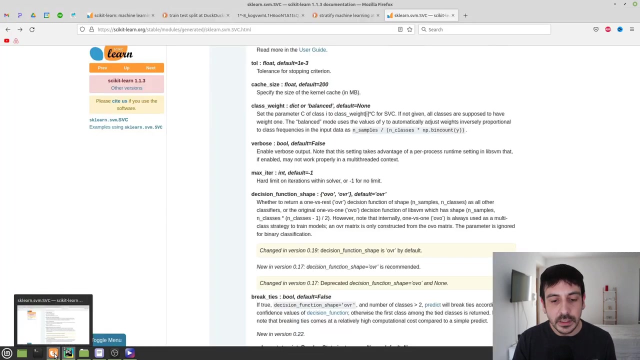 going to use and i'm creating this object, which is called parameters, which is a list containing- and this dictionary has only two keys: one one of them is gamma and the other one is c, and each one of these keys has a list of values. okay, now i'm going to show you the 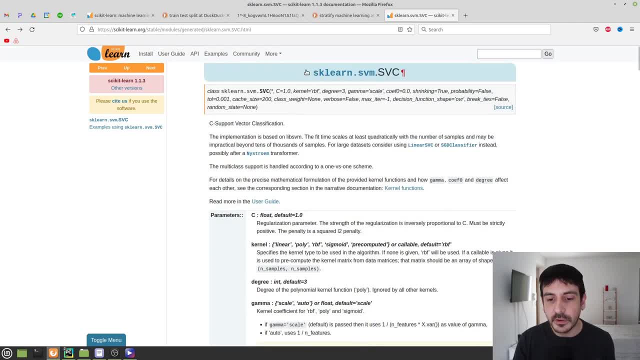 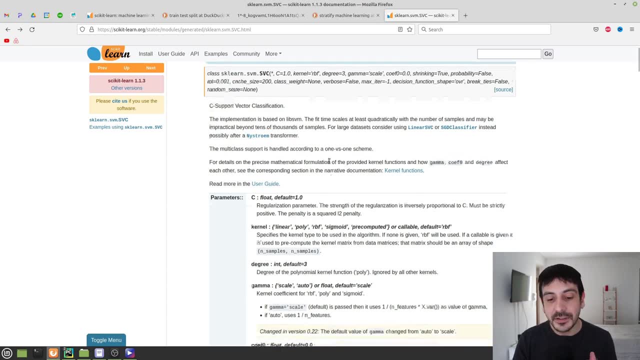 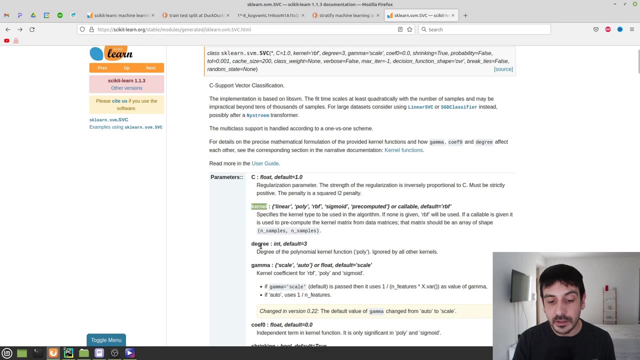 secret learn documentation. i'm going to, i'm going back to secret learn and i'm going to show you how the documentation looks like for svc, for the object we are using as our classifier, and you may notice all the different parameters we have in this classifier. we have c kernel degree. 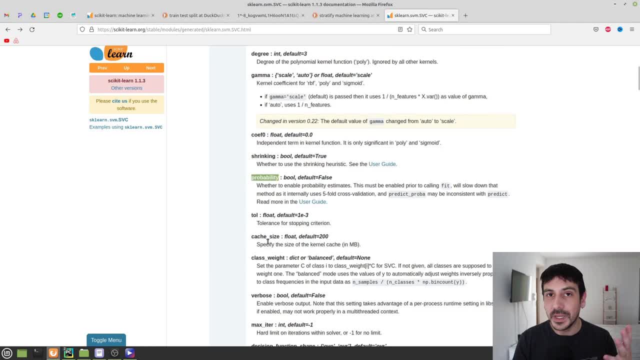 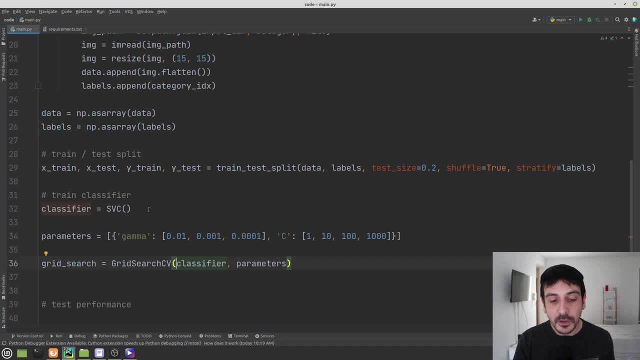 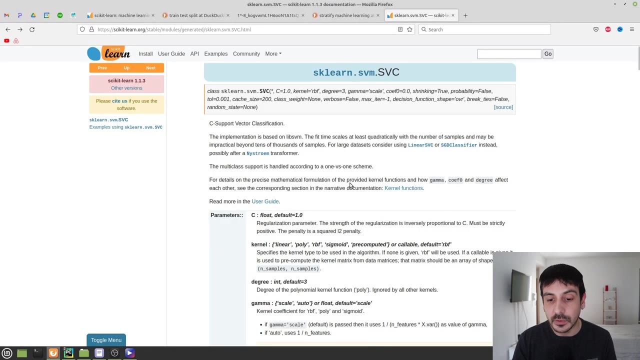 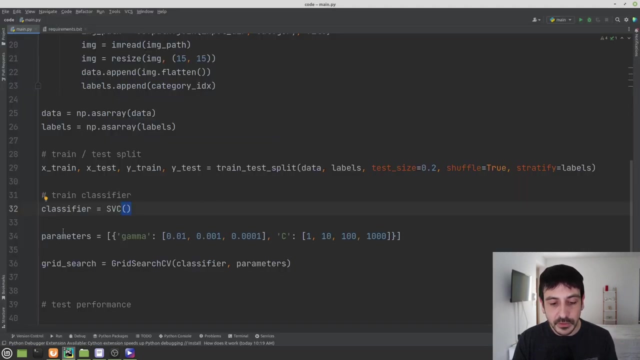 gamma, zero shrinking probability and many, many, many other parameters. we have many, many, many, many different parameters to choose from, but when we were creating our object, we are just calling this empty constructor. we are not specifying absolutely any parameter. we are just using all the default values for svc, okay, and you may notice as well that we are creating this. 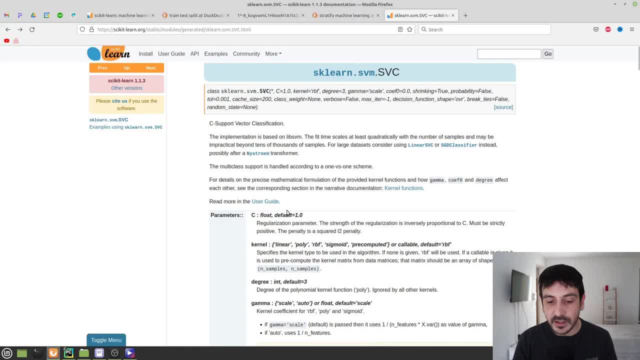 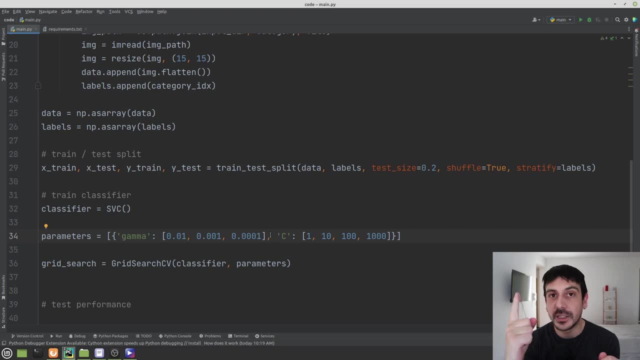 order object. and these two keys we are creating are exactly two parameters from our svc, from our object, from the object we are going to use as our classifier. so what we are going to do is we're not going to train only one image classifier, we are going to train many, many, many, many different image classifiers and we are going 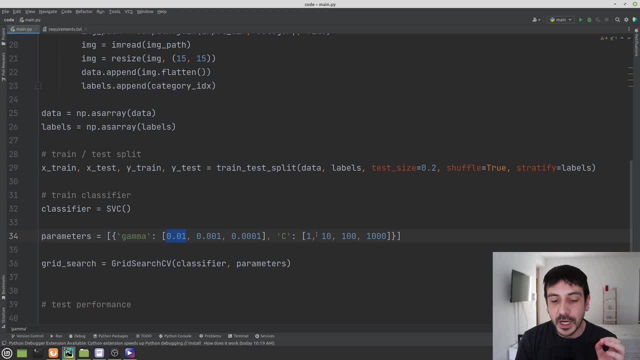 to train an image classifier for each one, for each combination. we have for c and gamma. so we have three values for gamma and we have four values for c. this means we are going train 12 image classifiers, right? the way this process is going to work is that we are not going. 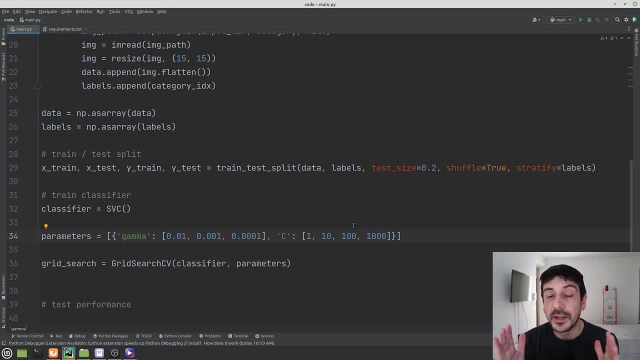 to train only one image classifier, but we are going to train many, many, many and as many as different combinations we have for c and gamma. in this case, we have three values for gamma, four values for c. three times four it's 12. so we are going to train 12 image classifiers. that's the. 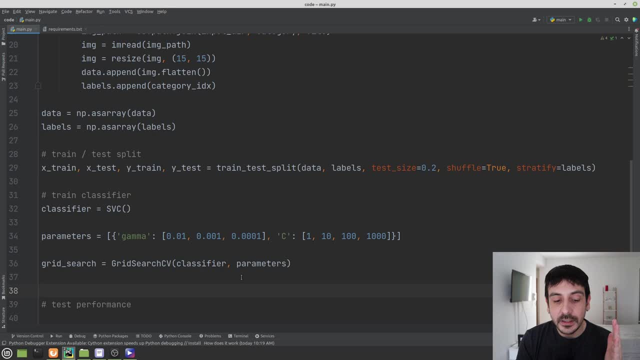 process we are going to take in this tutorial and the the. the way it works is that we are going to choose the best of all of these different classifiers. we are going to train so, and the way we are going to do this training, the way we are going to train as many classifiers as once- 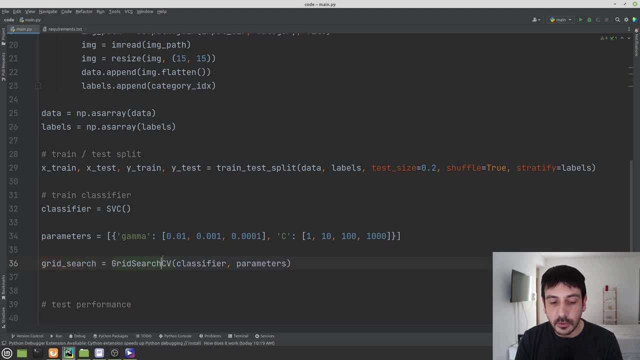 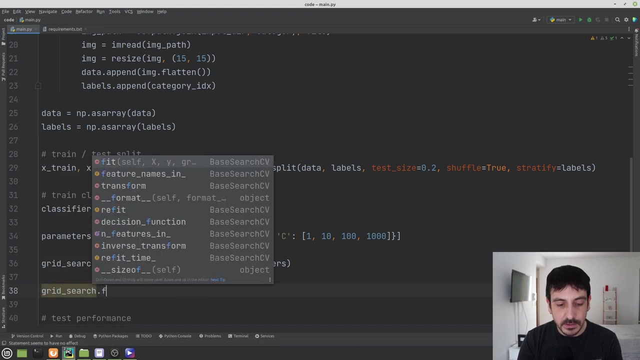 at once is by calling grid search, by calling this or object i have specified over here. so this is how we are going to use it. i have already defined this grid search and then the only thing we are need to do is to call grid search dot fit, and i'm going to input x train, which is my training set. 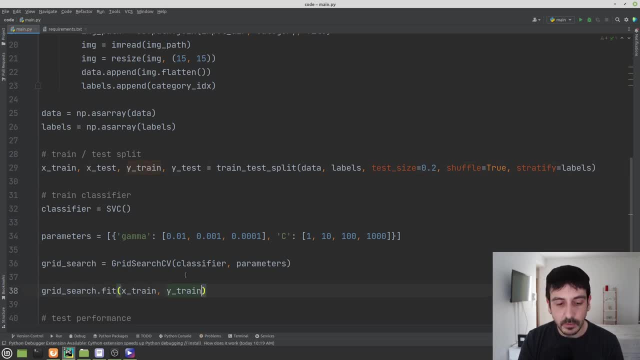 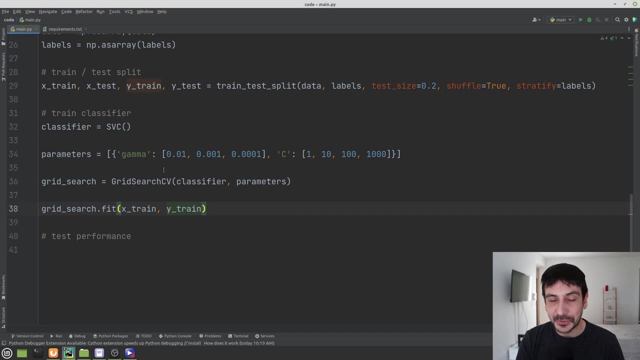 and then white train, which is, which are the labels of our training set, and that's pretty much all. that's pretty much all in order to train our image classifier. that's pretty much all to train all these 12 image classifiers. right, let's see what happens when i press play. now, remember the way. 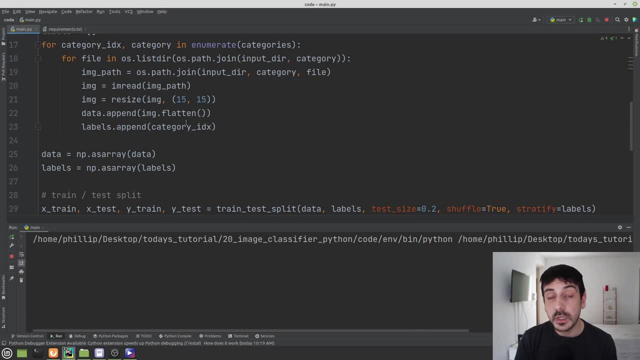 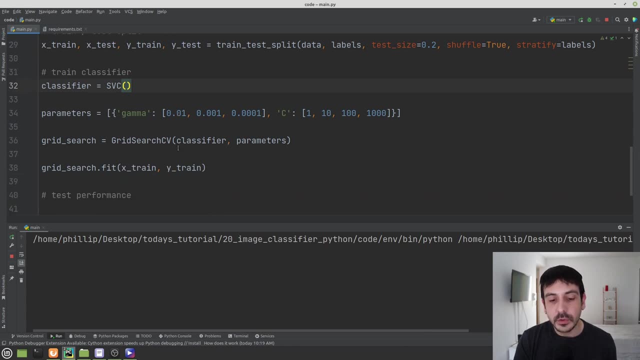 this works is that we are loading the data first, and this is going to take a few minutes because it's a lot, a lot of data, these are a lot of images- and then we are taking this process now. the training also takes some time because, remember, we are training many, many, many, many different. 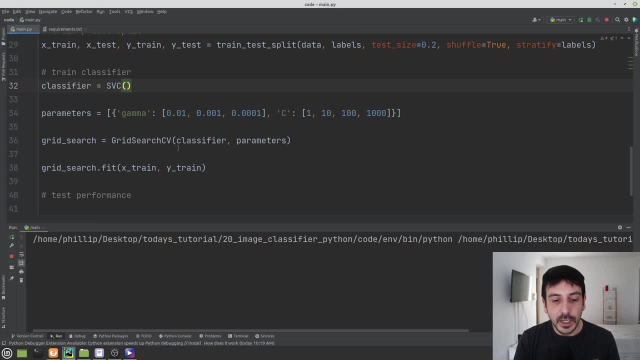 classifiers. so this is going to take some time. so i'm just going to wait a couple of minutes and i'm going to see if the training is going to be useful. i'm going to start now and i'll see if something happens or if the execution is successful. 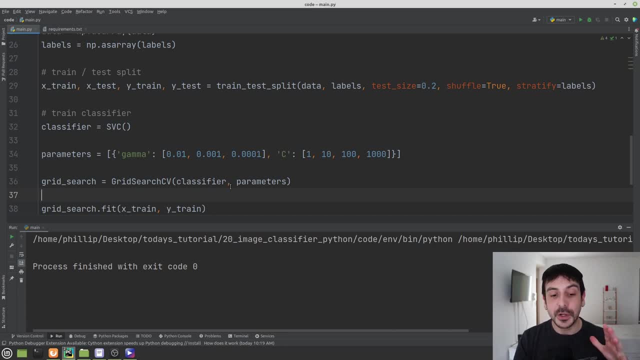 Okay, so the execution is now completed. We don't have any errors, so we can continue, And this was the third step in our four steps process. This means we are pretty much there. The only thing we need to do now is to test the performance. 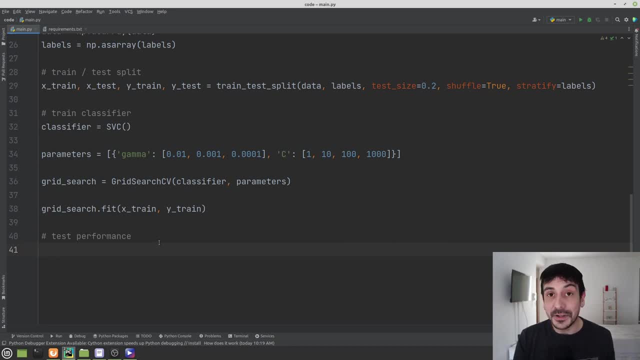 of the model we trained, but we are almost there. We have almost completed this process And, most importantly, we have already trained our image classifier. Our image classifier is now trained. The only thing we need to do now is to test how it performs. 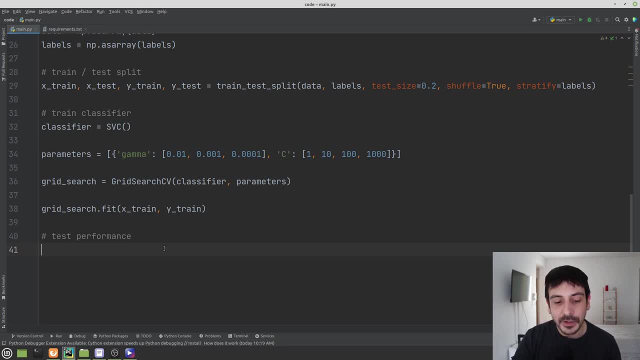 to see if we can use it or not. Okay, and this is how we are going to do. I mentioned that we were training not only one image classifier, but we are training 12 different image classifiers, one for each combination of C and gamma. 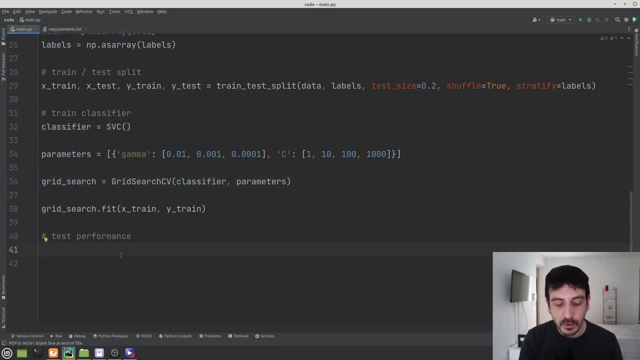 So we are training many, many, many different classifiers, And the way we are going to select one of all of these image classifiers is by calling a member of GridSearch, which is called gridsearchbestestimator underscore. So by calling this member, is that we are going to get? 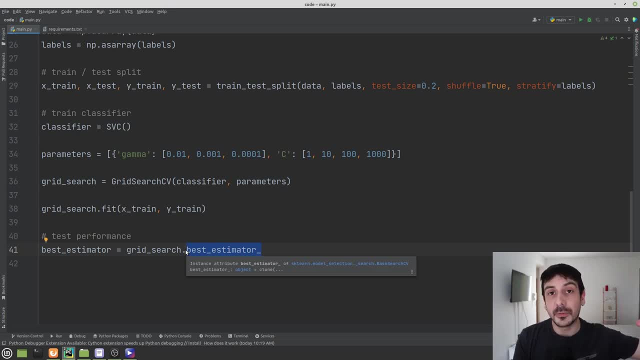 the best of all the different image classifiers that were trained. right, We are training 12 different image classifiers and we are just choosing the best one. And the way we are choosing for the best one is by calling this member of GridSearch. That's basically what we are doing. 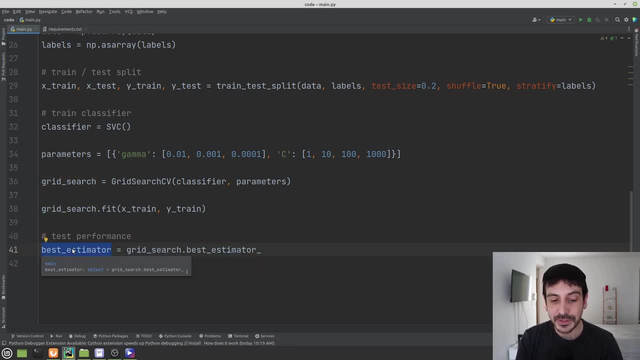 So this is our model, This is our classifier bestestimator. This is our model. Now let's see how it performs. Let's see if it's really like a good classifier. Let's see what's the performance of this classifier on our test data, on the data we have created. 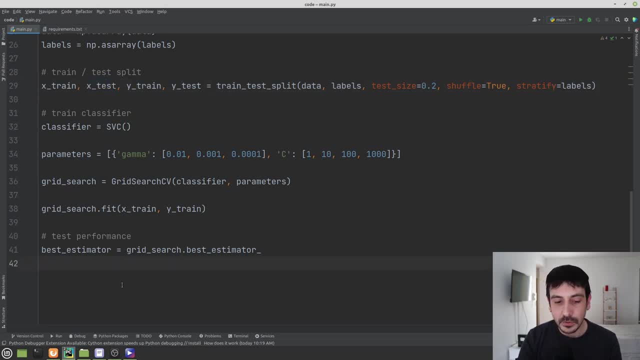 in order to test the performance of this algorithm. So what I'm going to do is to call bestestimatorbestestimator And I'm going to input my test data. So I'm going to input X test And I'm going to call the output from this prediction. 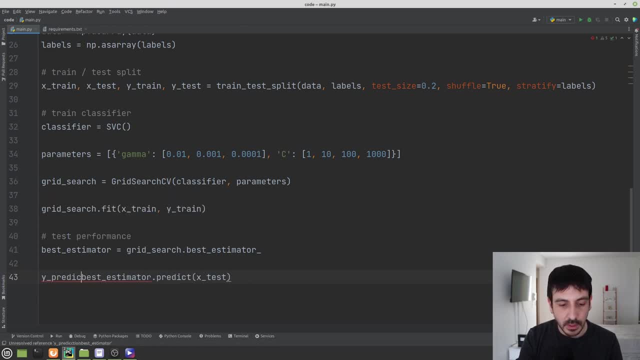 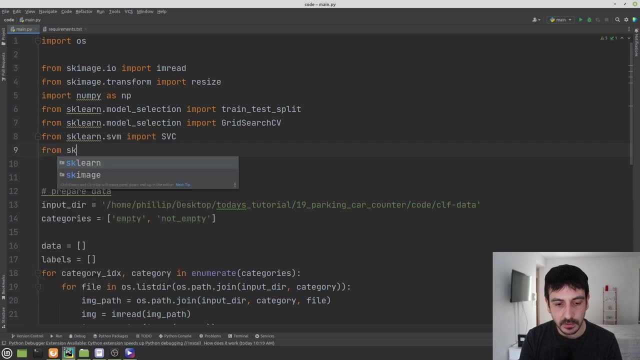 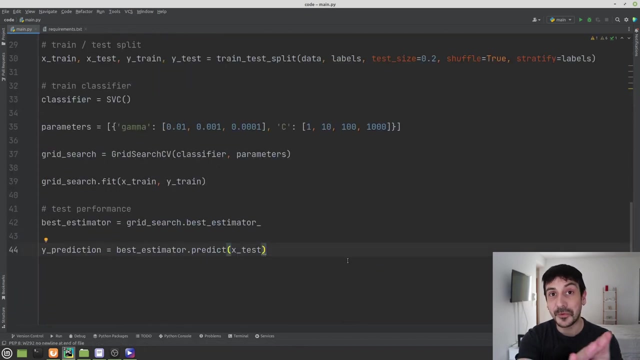 Y prediction right. And then I need to import another function which is from sklearnmetrics, import accuracy score And let's see what's our performance. And I'm going to make a print, I'm going to define another value, which is score. 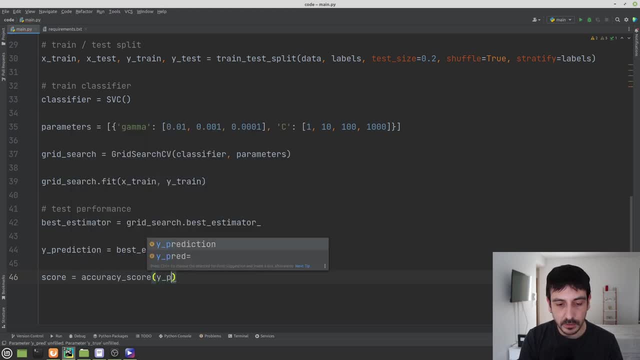 And score will be accuracy score, Y prediction and Y test. right, I'm taking these, which are the labels of the test set, And I'm just comparing against our predictions And now I'm going to print something like: I'm going to format these super, super nicely. 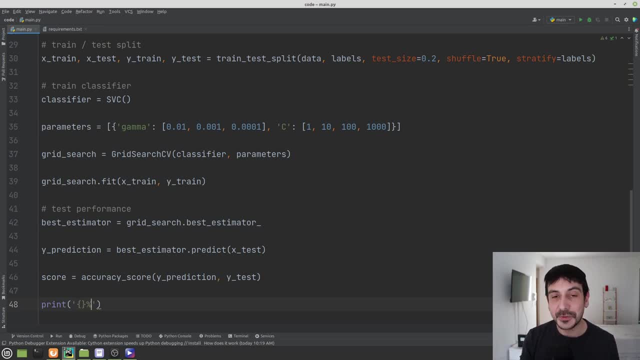 So we get like a very clear measure of how well this performs. So I'm going to express this as a percentage And I will say something like of samples were correctly classified, something like this. And this will be format string score: times 100, right. 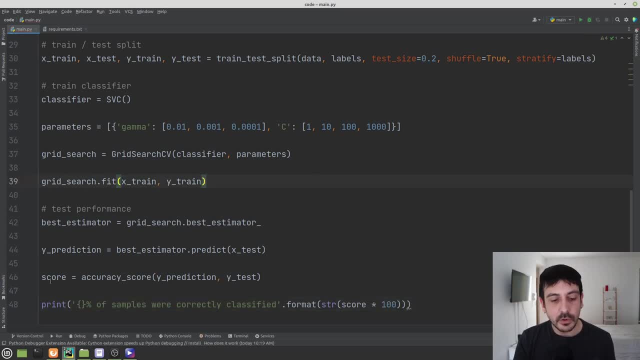 Because score is going to give us a number which ranges between zero and one And it's going to be a measure of our score, of how accurate our classifier is on the test set. Now, this is a value between zero and one. 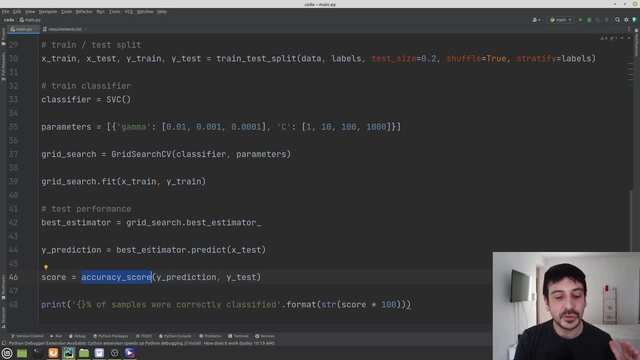 and it's very, very useful And that contains absolutely all the information. But what I'm going to do is just reshaping. We're going to do like a reformat of this number into a percentage Right, Because it's going to be much, much cleaner. 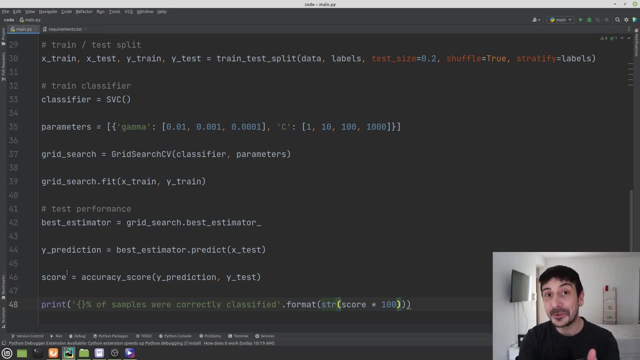 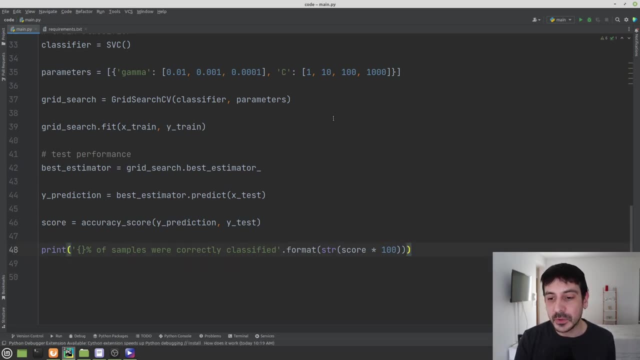 in order to see how it performs. And all I have to do now is to execute this code again And let's see what happens. Let's see what's our performance. So I'm just going to press play and I am going to wait a couple of minutes. 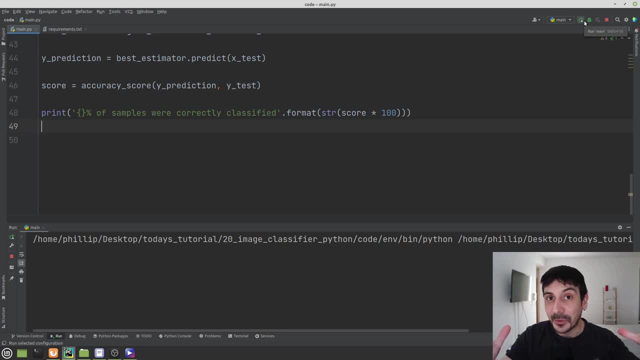 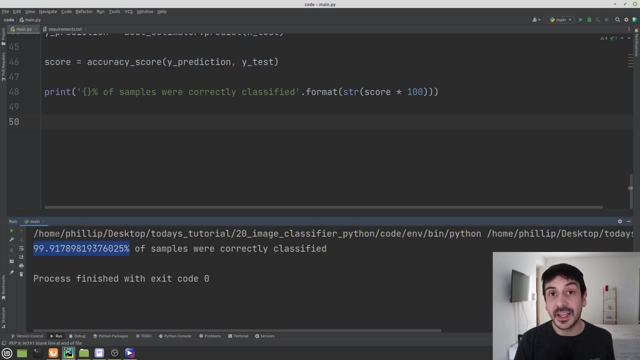 just like before, And I will come back with our results. Let's see how it performs. The execution is now completed And this is the accuracy we got with the best estimator from all the different image classifiers we trained. We are getting a 99.9% accuracy. 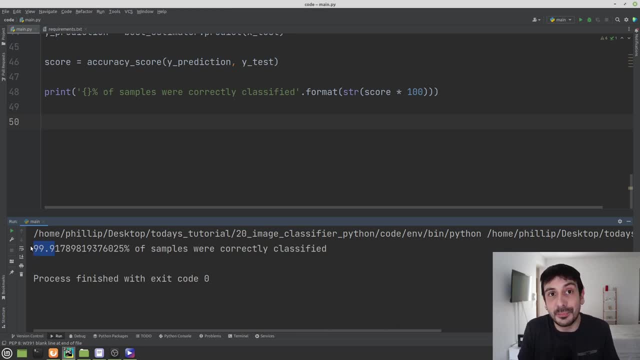 This means that this is absolutely perfect. This is a pretty much perfect classifier. A 99.9% accuracy is like a super, super high performance. It's like a very good performance, So we can definitely use this classifier later on. We can definitely use this classifier. 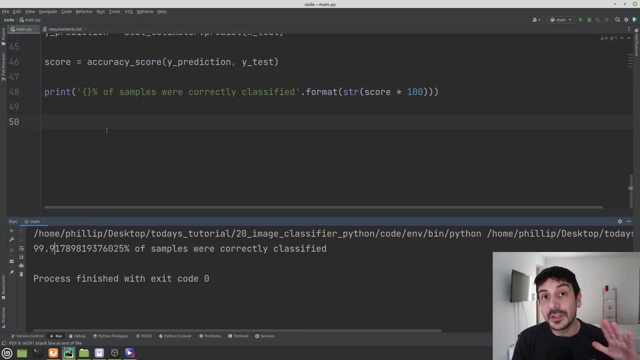 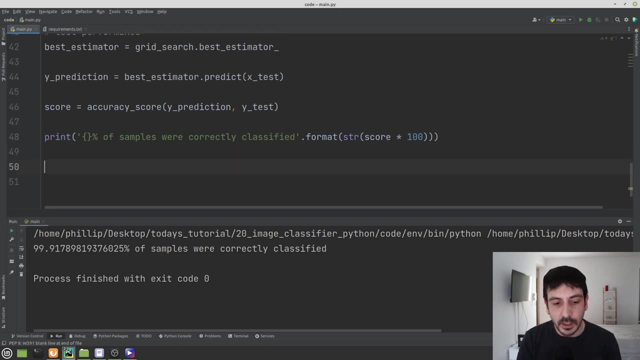 in order to use it in our project. So the only thing we need to do next, the only thing we have to do now in order to complete this tutorial, is to save this classifier, to save this model, because we want to load this model from another project. 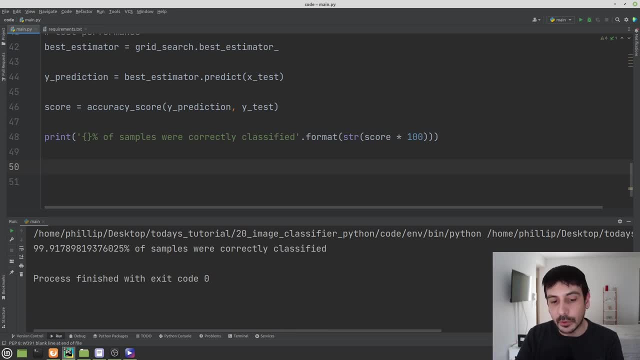 or we want to load this model in a different code or in a different whatever, from a different location. We definitely want to save the weights, or we want to save exactly all the information which is related to this model, so we can use it later in a different project. 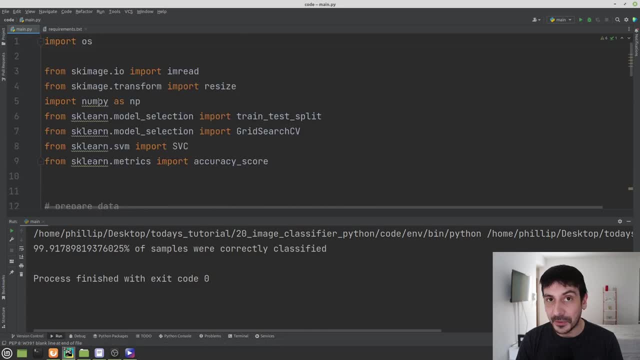 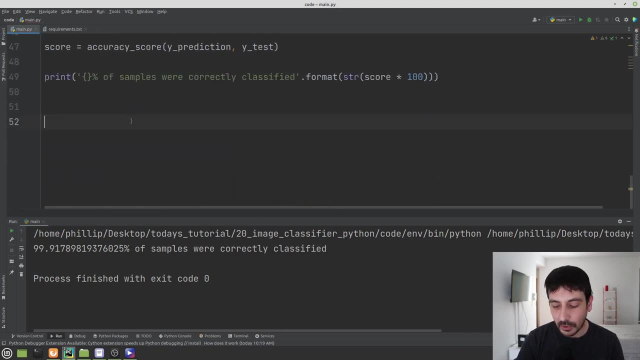 And the way we are going to save this model is by using pickle, which is another Python library. So I'm going to import pickle and then I'm just going to call pickledump And I'm going to specify the model I want to save. 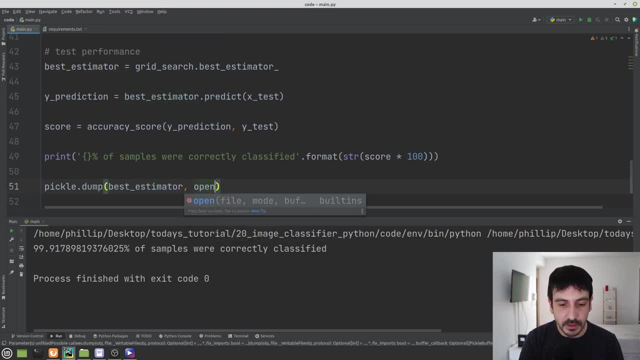 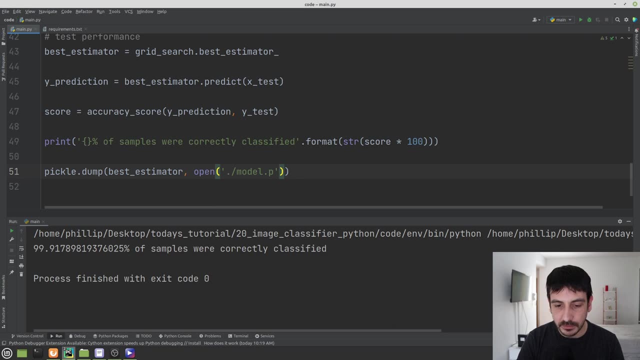 the object I want to save, And also I need to specify the file, which is going to be something like modelp, And then I need to open this file as wb. Okay, and that's going to be pretty much all, in order to save our model.